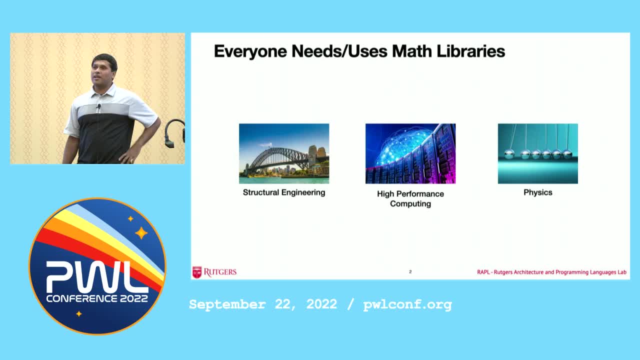 these math libraries contain. These math libraries contain elementary functions, which are functions of a single variable involving addition, multiplication of trigonometric functions, logarithms and polynomials. They're used everywhere, So it's like plumbing right. Everyone relies on it. 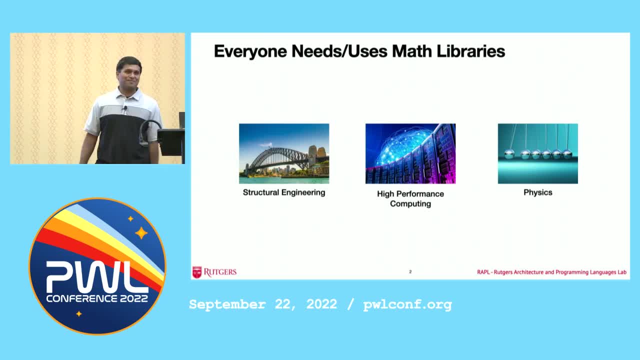 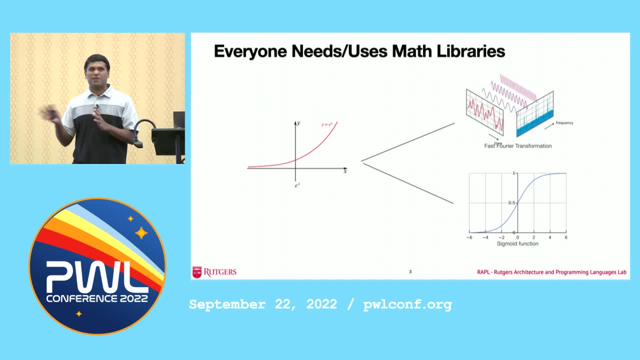 No one worries about it- And you need a plumber. you have an emergency. So if you're using machine learning- e power x, sigmoid function, natural language processing, speech processing- you just had a talk on processing beats right Like e, power x plays a prominent role there, So it's all there. 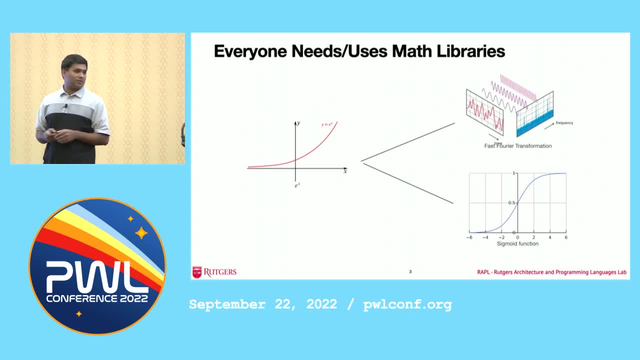 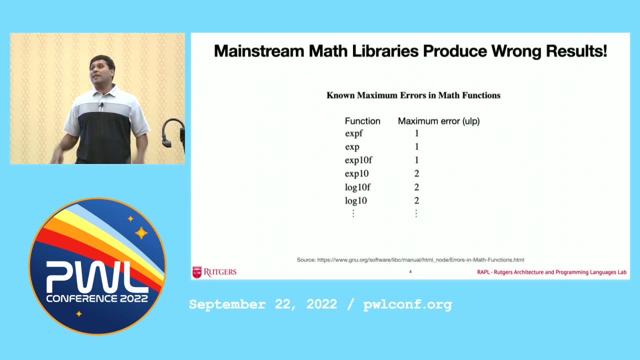 So, unsurprisingly, you have implementations for these functions. Where do you find them? In math libraries Like hyphen lm. when you compile your code, They're automatically included, But unfortunately they're all wrong. So I'll tell you what wrong means. So I come. 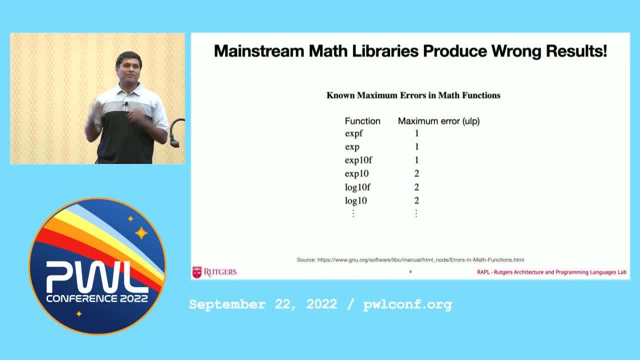 from a formal methods world. Like wrong means oh man. Everything is failing. So one of the issues with having wrong libraries is non-portability. You have your fancy GPU. you run your training model. it produces some results, You just port it to another nice. 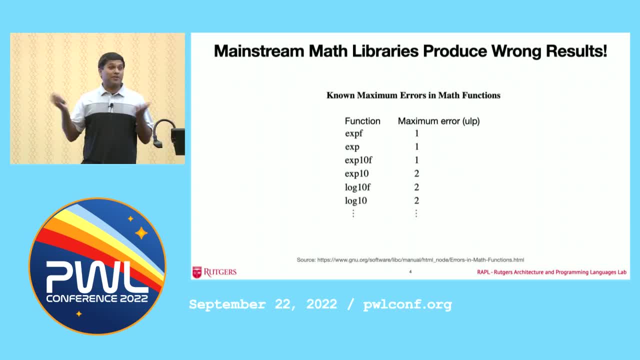 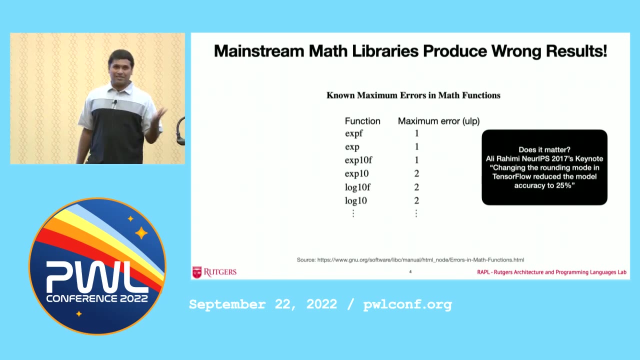 GPU that another company has brought up, you get totally full-bar results. Imagine, if you Imagine you are the developer trying to debug it. What nightmares you will go on Again. Santosh is another guy just talking about random things, right? If you don't trust me, there's a nice keynote by Ali Rahimi. he's a machine learning researcher. 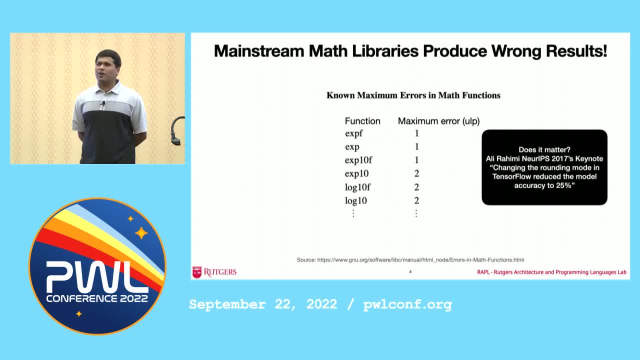 at NeurIPS And in the middle of the keynote he has a code. This is a production bug report filed by one of his team members. Oh, I changed the rounding mode in my training from round to zero. Why would anyone use round to zero? 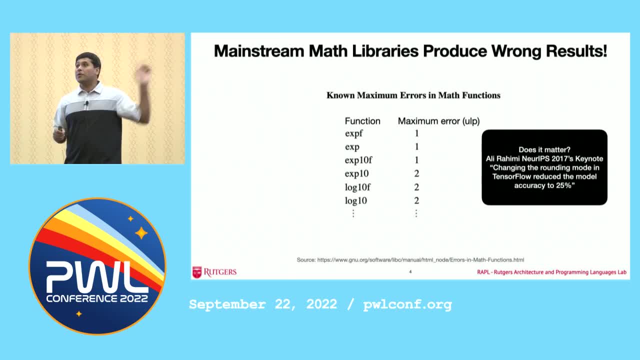 It's attractive for performance And accuracy dropped to 25%. The model had a reasonable accuracy- 85% or so- And now it's 25%, doing nothing, just changing the rounding. So this is where, like, if you want to care about portability, if you want to make your 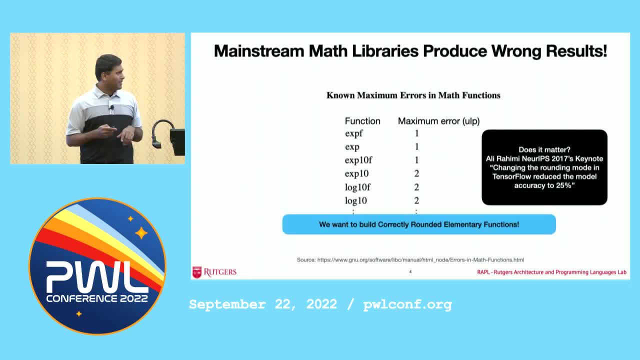 code robust. there's a lot of interesting things to do in this space. So effectively, we want to build correctly rounded elements And, as Zeeshan alluded to, I come from the compilers and formal methods world. You don't wake up one day and start working on numerical analysis, right? 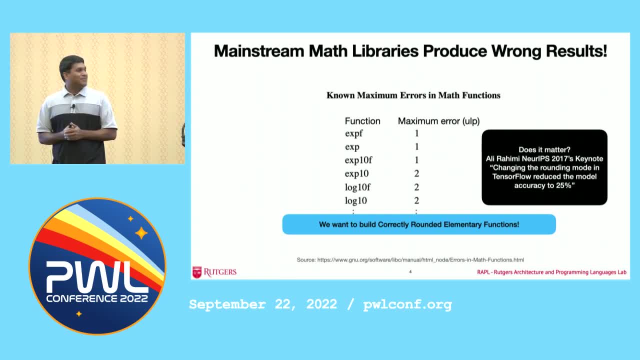 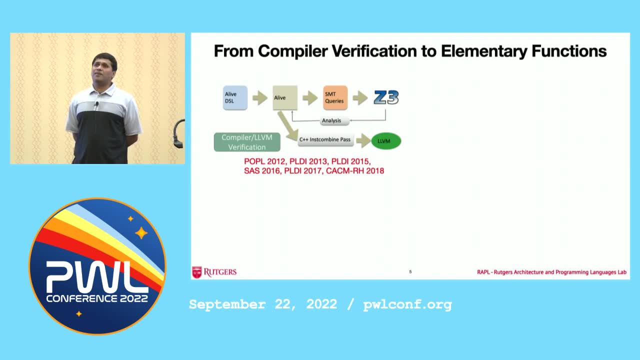 Let me tell you a story about how I got excited about this area. So about ten years ago we had been working on proving the correctness of compiler optimizations. Compilers are large pieces of software, million lines of code. everyone relies on them. 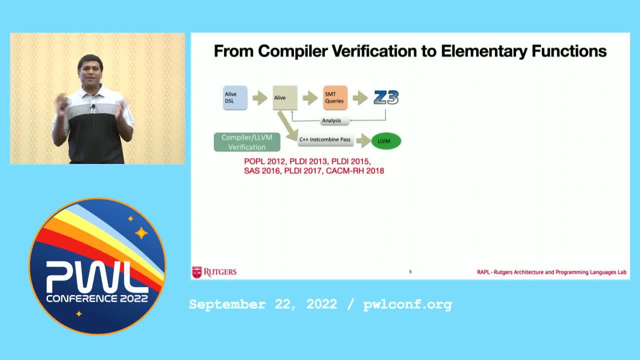 And there are bugs And it's a fact of life, Like bugs are always there. But you don't trust, you don't believe a compiler is wrong, right, Sometimes, if something is wrong, you just: oh, my code is wrong, let me fix it first. 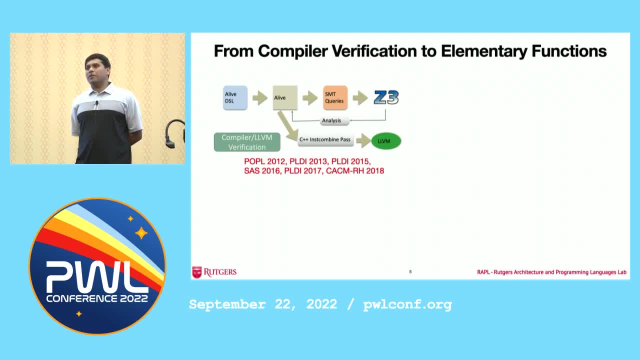 But compilers do a lot of crazy things and they're wrong. So we wanted to address it. We built formal semantics of the LLVM compiler in the Coq proof assistant in collaboration with my advisors at Penn, Steve Danzabek and Milo, and then we realized like it's very 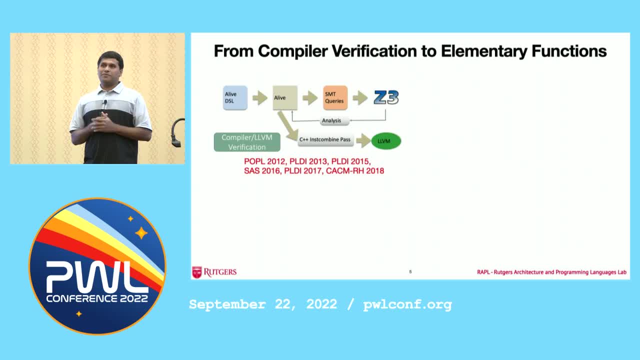 difficult to get traction from developers. So what did we do? So, in collaboration with my student and a few other collaborators at Utah, John Regehr and Nuno Lopez, we built this domain-specific language called Ally, So effectively. what was it? 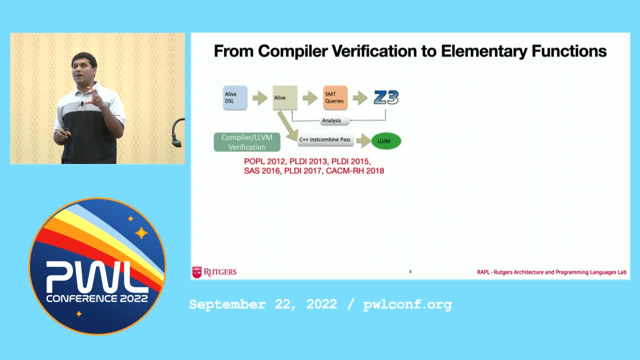 What was Ally? Ally was a small DSL where you would specify your optimization in this DSL and you would automatically prove its correctness using theorem provers- first-order logic theorem provers. We would generate SMP conditions. We would give it to Z3.. 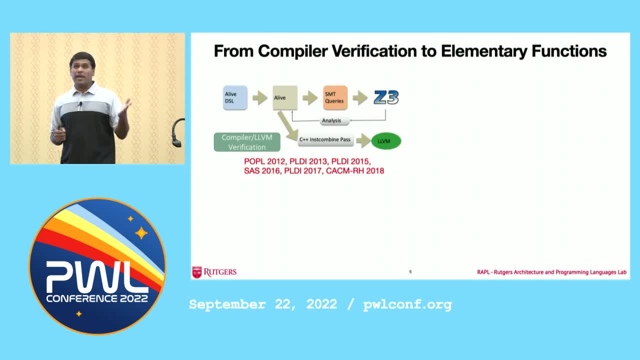 If it's correct, your compiler optimization is correct, And today a lot of many LLVM developers use Ally to check the correctness of new optimizations. Okay, So this was primarily like people of local rewriting rules And my student was like, okay, we were just focusing on integer optimizations. 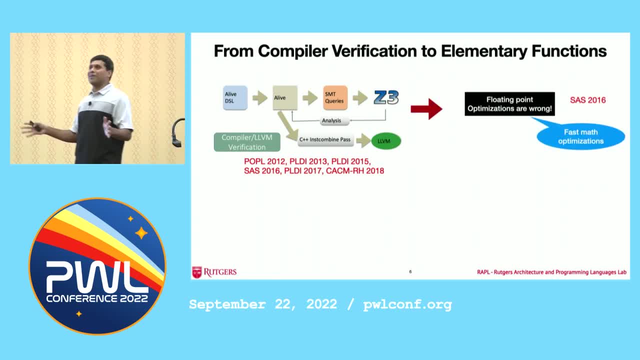 What about floating point? And compilers, like compiler optimizers, fall into two categories, right Like one. I don't want to do anything with floating point, I just want to say IEEE says this, I'll just do that. 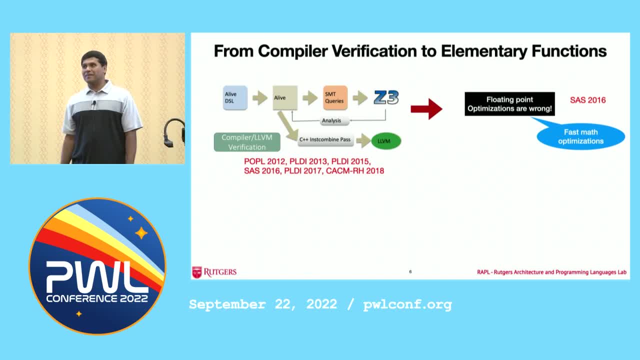 Even when they do that, they make mistakes. So we had a snippet of Ally called Ally OFP, where we wanted to check bit-precise optimizations. Is the value produced exactly bit-to-bit same? Okay And IEEE-compliant? 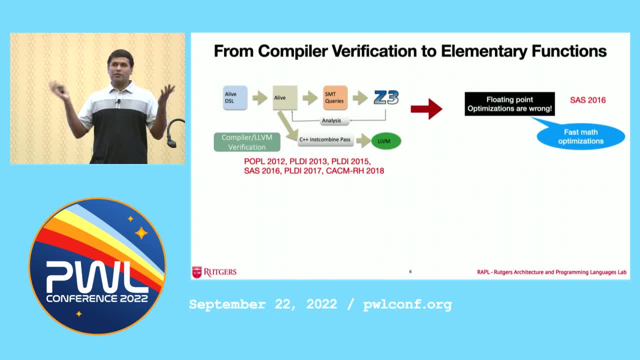 And we found bugs. And if you don't know floating point, there are two zeros plus zero and minus zero. And I found a bug. So I found a bug And what happened? And one of the LLVM optimizations was changing the sign of 0, OK. 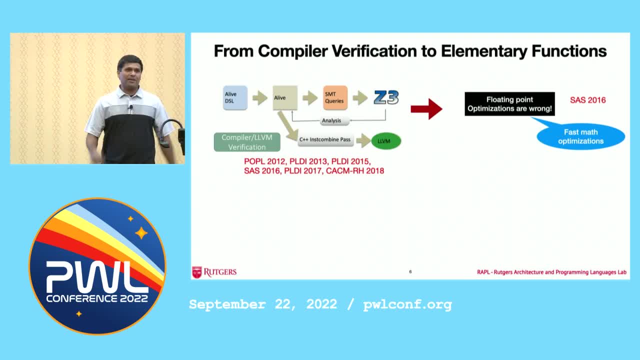 So my student told this to his lab mate and he said: who cares about the sign of 0?? But William Kahn, a Turing Award winner, has a nice article that says if you change the sign of 0, it causes discontinuities in branch cuts. 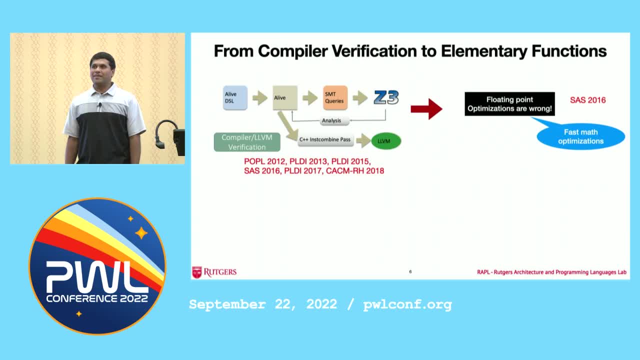 So we filed this bug. It was immediately fixed, OK. And then there are the second class of compiler optimization designers. They have this demonic mode called fast math, or I would call it incorrect math. OK, So what do they do? It considers any real identity as a floating point identity and optimizes code. OK. 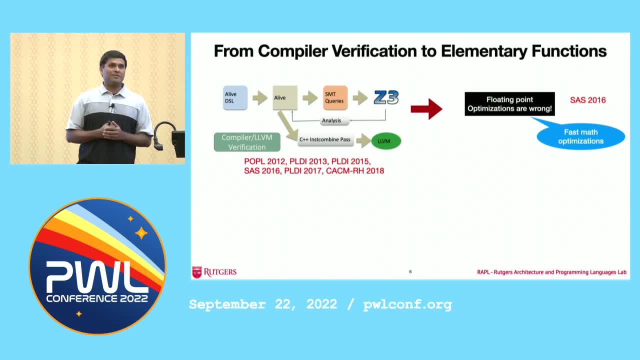 So associativity is not true with floating point OK. And when you invoke fast math, they say, oh, floating point, arithmetic is associative. It's very important. You should not blame them, because you can't do parallelization without associativity. 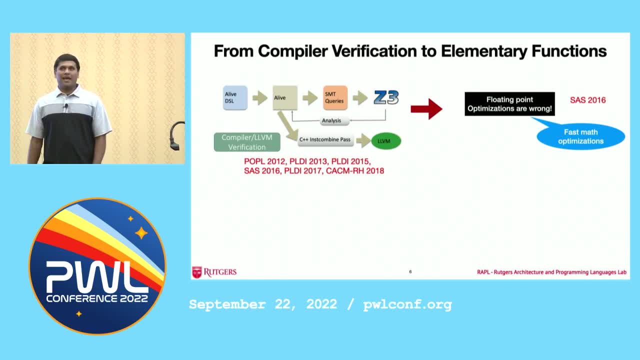 OK, So there is this fast math mode, And this is the advantage of having curious students, right? My student then was taking a machine learning course And he had a nice data set. He was learning some training algorithm, a support vector machine training algorithm. 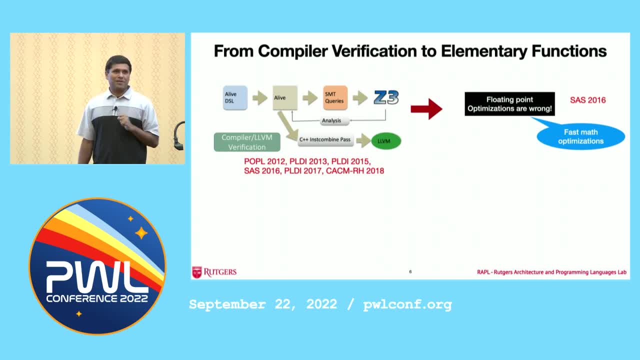 He implemented the algorithm in C++- He was learning- And then trained it on a curated data set. He got a reasonable accuracy And then, out of curiosity or magic I would say, he turned on fast math optimizations And the accuracy tanked significantly, doing nothing, 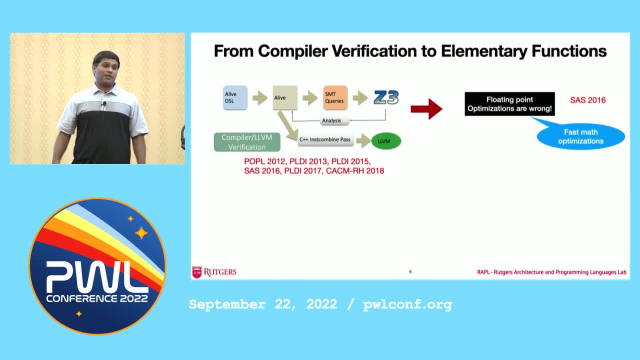 Training for the same number of iterations, same amount of time. the accuracy drops And he wanted to debug it. And, as I said, what is the issue with portability? Small errors getting magnified right. So debugging is a nightmare. 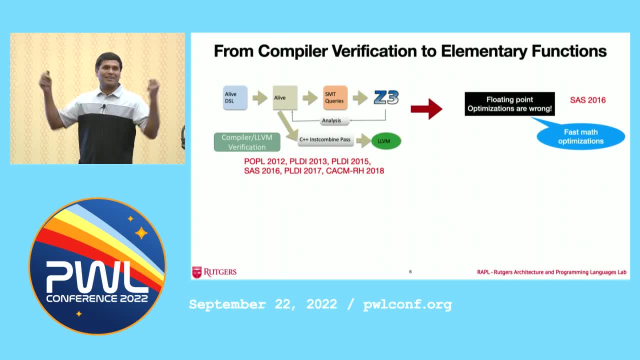 OK. So we looked around, Who can help us? Right Like, are there debuggers available? There was none, So we built our own. OK, So what debugger would be useful? So we said let's do a shadow execution. 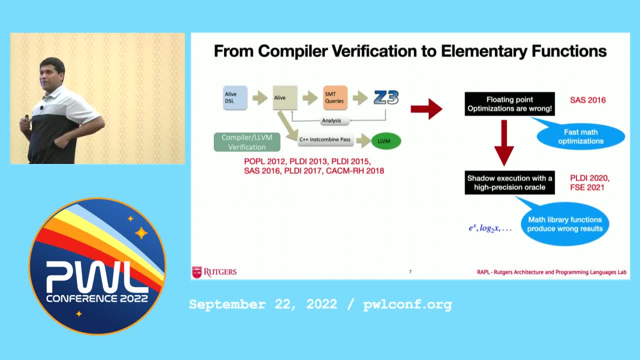 What do we do? We have your regular floating point program. You have your another program where we execute it with real numbers, simulated with MPFR, which is very slow. But we do log step execution with real numbers And we compare. 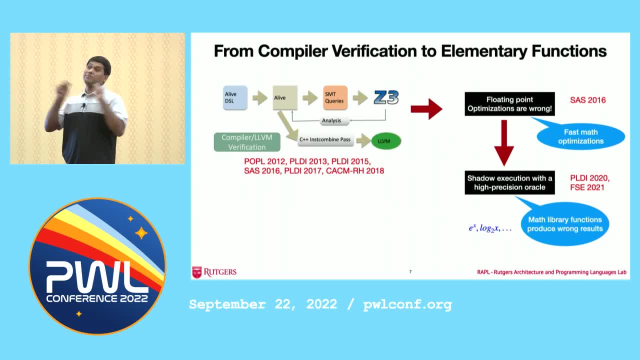 We do the Oracle program And we compare And the floating point program diverges. OK, And it turned out the divergence happened in the math libraries You would call a math library and it produces a very small error in the result And it gets amplified with cancellation and various other things. 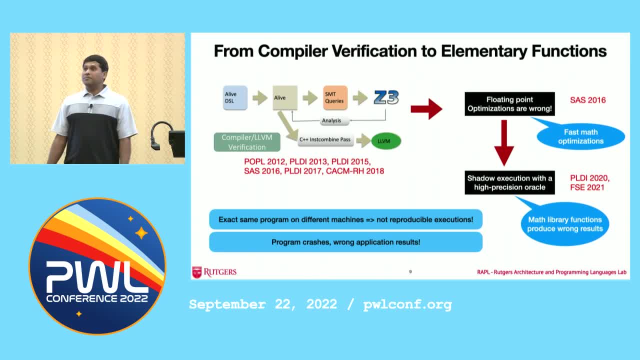 The end result is crashes. OK, And we had like lots of nightmares debugging it, reproducing the same bugs and other aspects of it, OK. So this is what got us excited about looking at this problem. OK, Math libraries are producing wrong results. 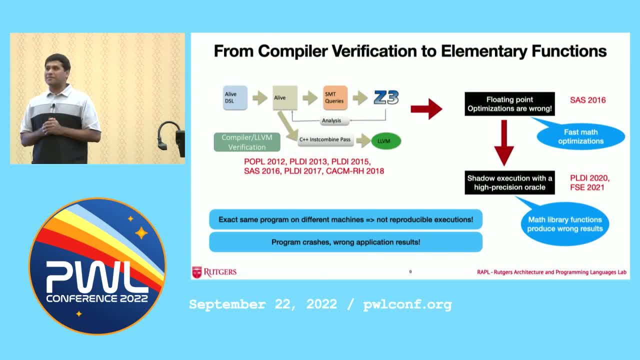 This is not a new problem. Why aren't people producing correct results? OK, So now, what is a correct result? I've been talking about wrong results. correct results. What is a correct result in the context of a floating point? Right? 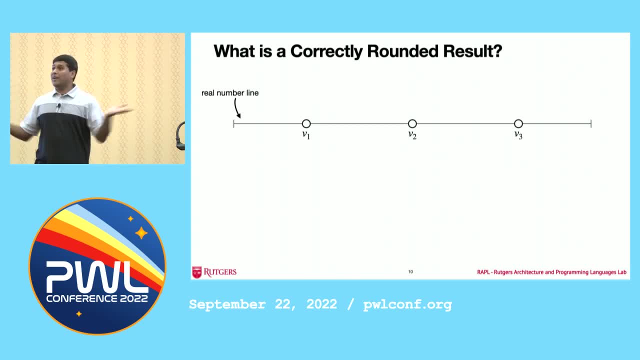 You have a number line. Here I'm showing you the number line. You have infinitely many real numbers. You cannot represent everything with floating point. You only represent finitely many real numbers with a floating point representation, which is a finite precision representation. 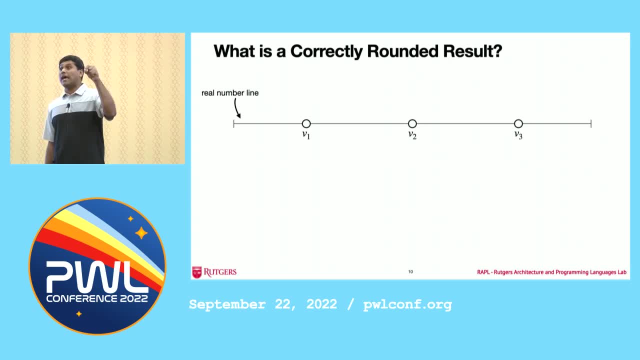 So here v1, v2, v3 are values that are exactly representable with a floating point. OK, And now you call an elementary function a math library function, lan of x, right, So it's called elementary because it produces an irrational value. 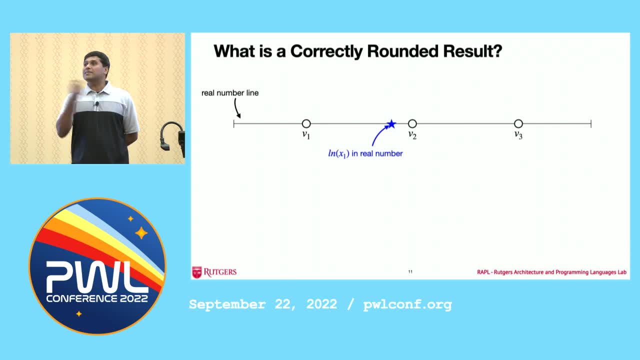 Most likely, in 99% of the case, this value will not exist. It will not be exactly representable in your floating point representation. So now, what do you do? You need to do round the result to the nearest floating point value. 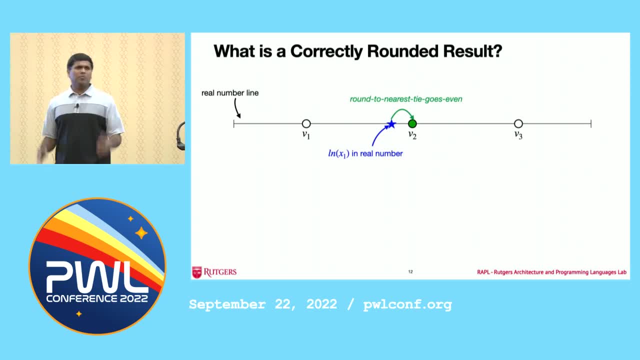 And there is a rounding mode. It specifies how you do the rounding. The most commonly used rounding mode is round to nearest twice to even OK. So what did you do? You take your favorite algorithm for approximating lan of x, do it with real numbers and then 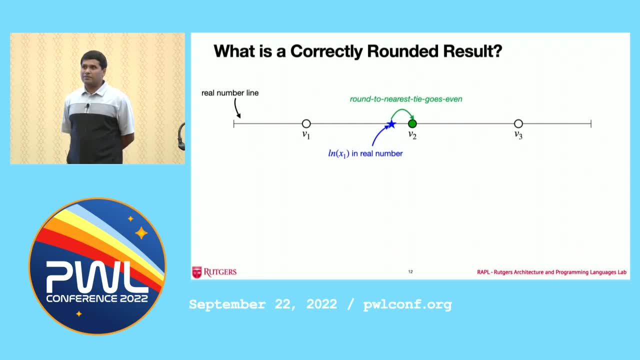 do the final rounding to get the floating point result, And here v2 is the correctly rounded result. OK, If your library produces the correctly rounded result for all inputs, it's a correctly rounded library. OK, So why is this useful? 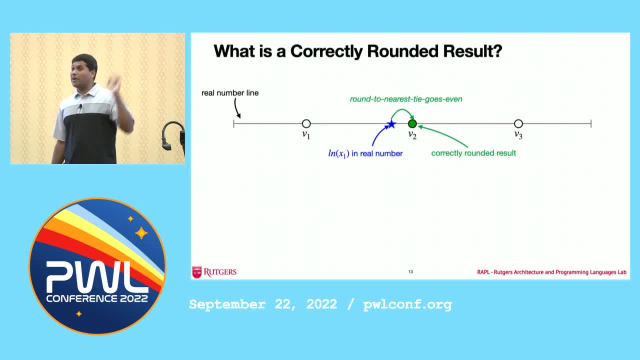 It is useful because it enhances portability, Like, for example, long ago when IEEE standard wasn't around. every hardware vendor had a standard. They had their own implementation of floating point. Porting code across multiple processors was just a nightmare. 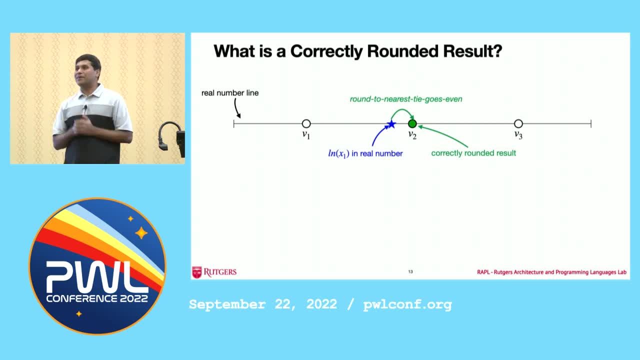 OK, So by standardizing it you can make the life of developers easier. So ideally we want a correctly rounded library. Unfortunately, the conventional wisdom is generating correctly rounded libraries is very expensive And that's why IEEE standard does not mandate correct rounding for elementary functions. 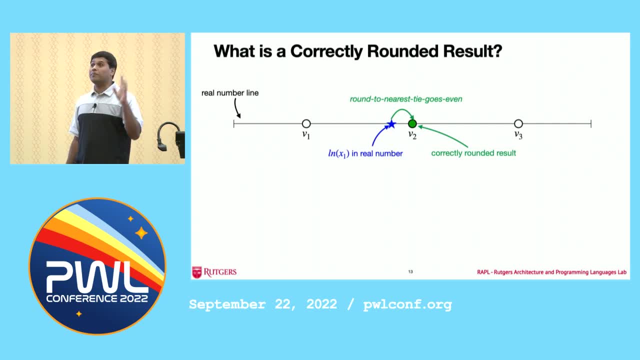 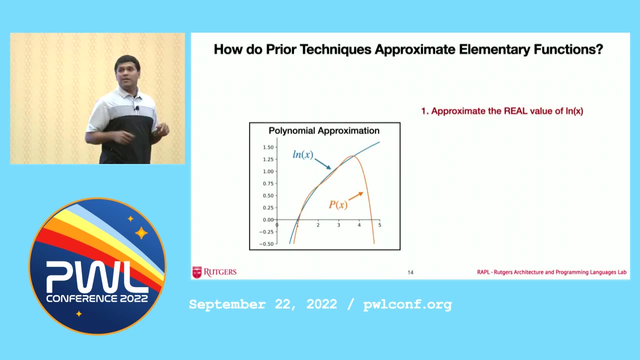 It's just a way to make it easier. It mandates correct rounding for primitive operations: addition, multiplication, subtraction, division and square root. OK, So now why aren't existing approaches producing the correctly rounded result? So even before you go there, we need to identify. how do people approximate elementary functions? 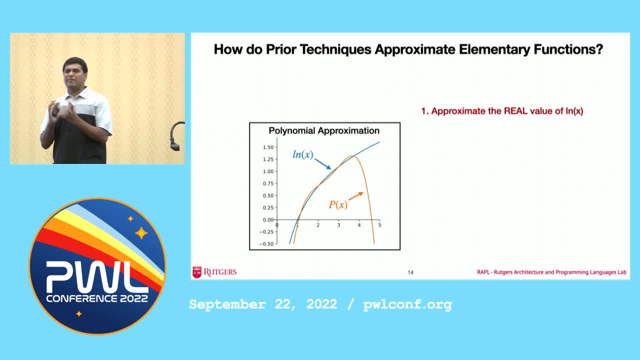 OK, So this is where, like, you'll have a brief taste of real analysis if you have taken it, but you don't need to know anything to understand the talk. OK, So everyone approximates elementary functions with polynomials. So there are classic results from real analysis: Weierstrass approximation theorem, which says: 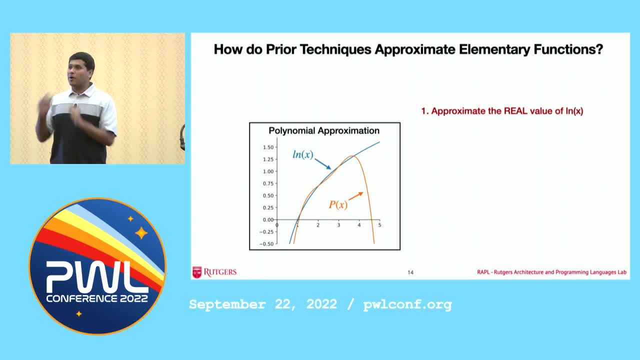 that if you have a continuous real valued function over a small domain, you can approximate it with a polynomial OK. So everyone approximates the real value of f of x. As I show in the slide, such a polynomial approximation is feasible only if you do it. 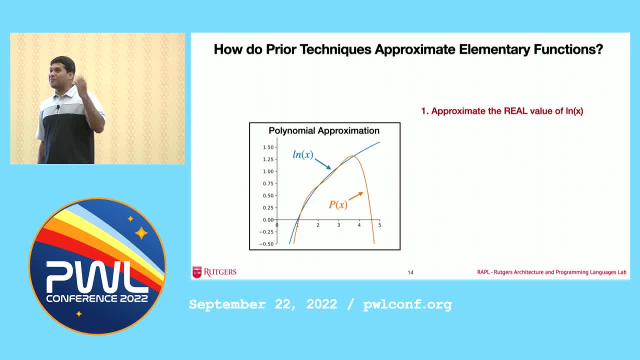 over a small domain. And what is the range of a 32-bit floating point, 2 to the power of 128 to 2 to the power of minus 149.. And you cannot do polynomial approximation over such a large domain. So the first step in any elementary function implementation is to do range reduction. 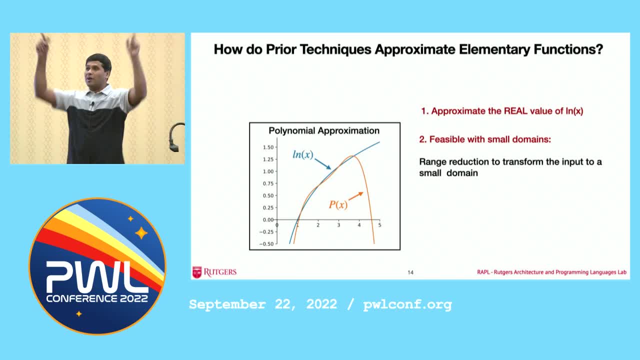 So what is range reduction? You're reducing an input which belongs to the domain 2 to the power of 128 to 2, to the power of minus 149, to a smaller domain. What should this smaller domain be Ideally like for large domains? 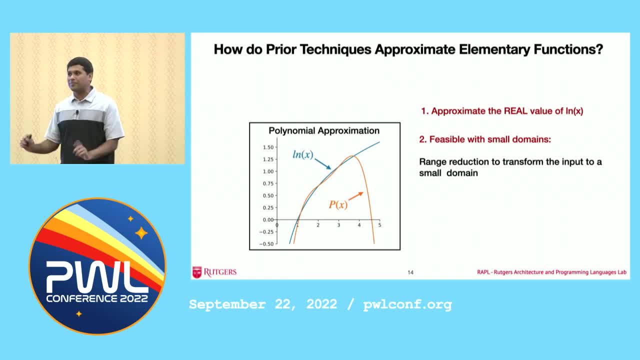 And it should be 1 to 2, or like 1 to 1.33 or something. OK, So how do you do this? So you use mathematical properties of logarithms or the elementary function of interest, and you do this. 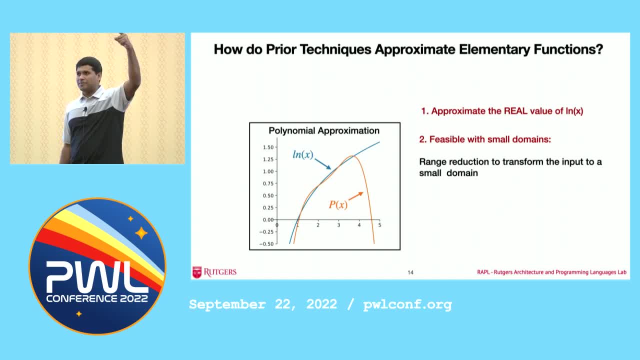 OK, So you approximate the real value of f, of x, and then you reduce the input to a smaller domain, And now you do polynomial approximation over the smaller domain for the reduced input And eventually you get the result for the reduced input. 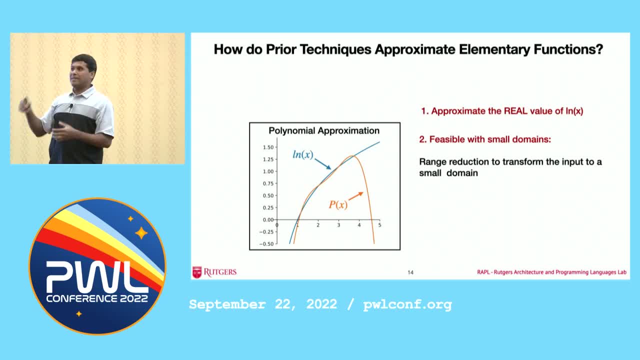 What do you do? What do you need to do? You need to compensate the result that you get, to produce the result for the original input. So this last step is called output compensation. So if you forget all the jargon, like, the thing you need to remember is: everyone approximates. 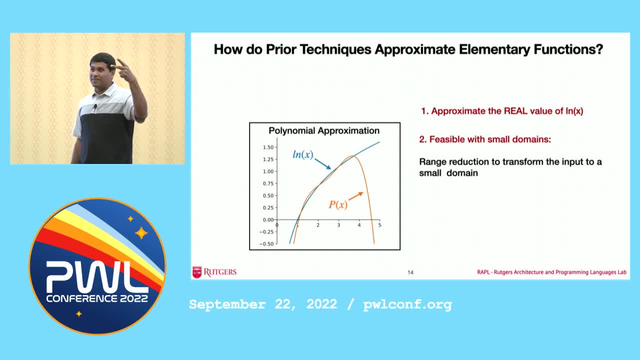 the real value, And then they do range reduction, And then they evaluate the polynomial over, create a polynomial approximation over the small domain, And then they compensate the output, which is called as output compensation. All these four steps are done using floating point. 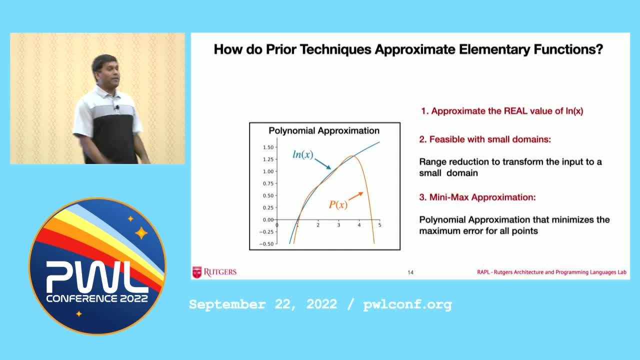 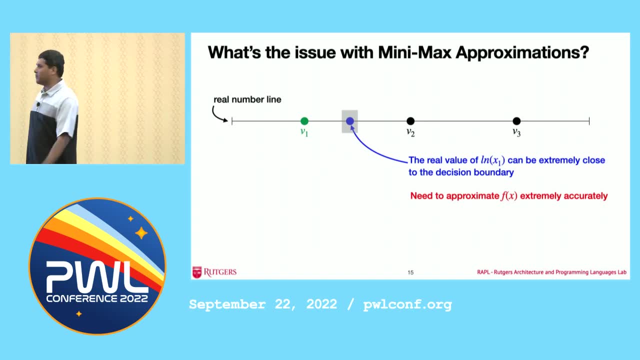 OK, So they're going to have some error. OK, So now why do they produce wrong results? So I'm going to pictorially represent what happens with an existing approach. Let's say, the real value of your elementary function is very close to the rounding boundary. 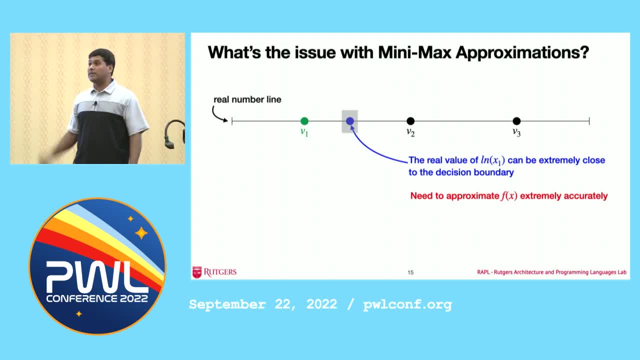 OK, In this case, in the slide, v1 and v2 are two representable values in your floating point representation. So what is the rounding boundary With respect to round to nearest ties, to even? it's the midpoint. If a real value is very close to the midpoint, any small error that you will have will make. 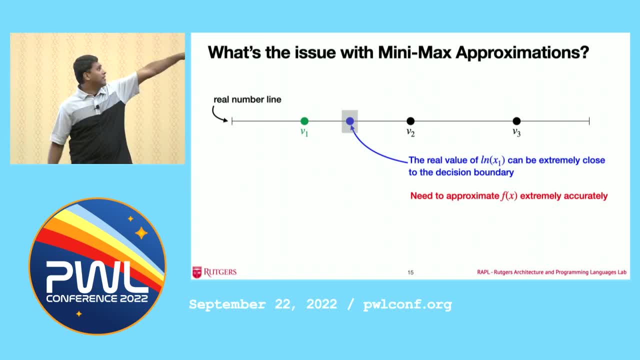 it produce a wrong result. So the freedom that the polynomial generator has is the gray box that I show in the slide. OK, So now recall What did I say You have to do: range reduction, output compensation and polynomial evaluation in floating point. 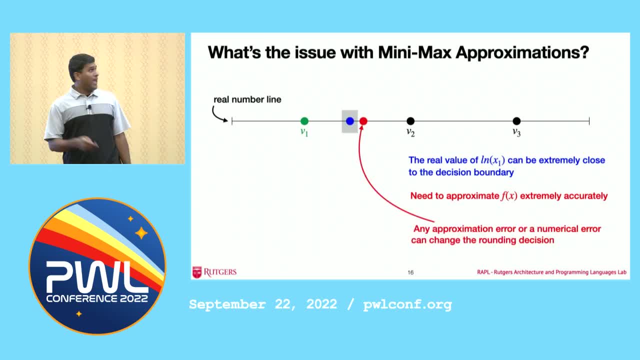 All those is going to have some error. OK, So any such error is going to push the value outside and eventually resulting in wrong results. OK, So the key takeaway I want to remember is: everyone is approximating the real value of f of x. 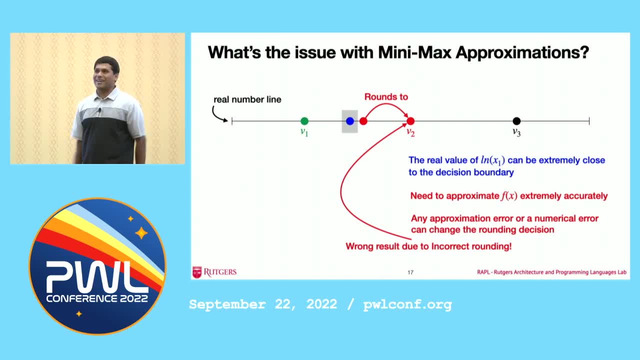 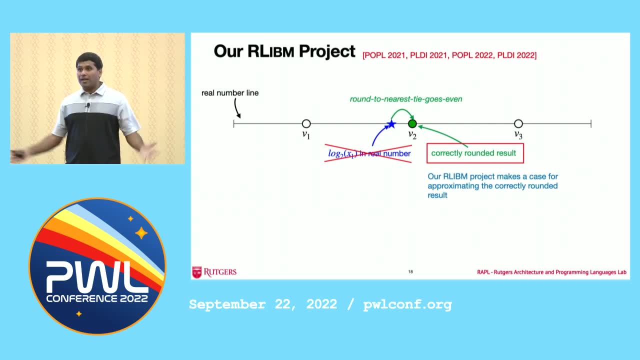 So our epiphany or our key insight is: why are we approximating the real value? In the RLibm project, we make a case for directly approximating the real value of f of x. So what is the real value of f of x? 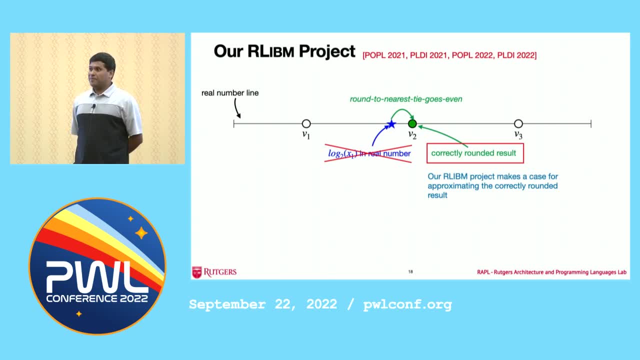 We are directly approximating the correctly rounded result. Why, You are not worried about the real value. You only care about the correctly rounded result. Directly approximate the correctly rounded result. Well, you're thinking man. are you fooling us? 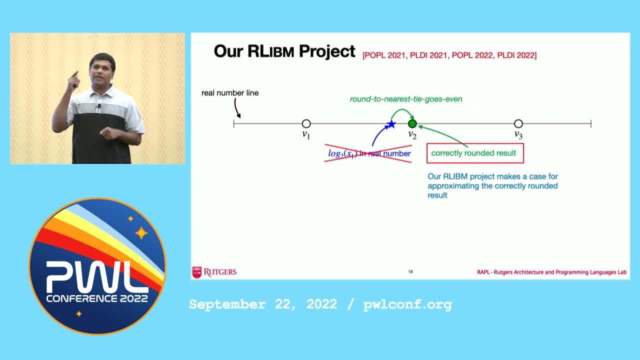 You said you want to approximate the correctly rounded result, But you know the correctly rounded result only when you know the real value. How do you know the correctly rounded result? So our key insight is: when you cannot solve a really complex problem, split the problems. 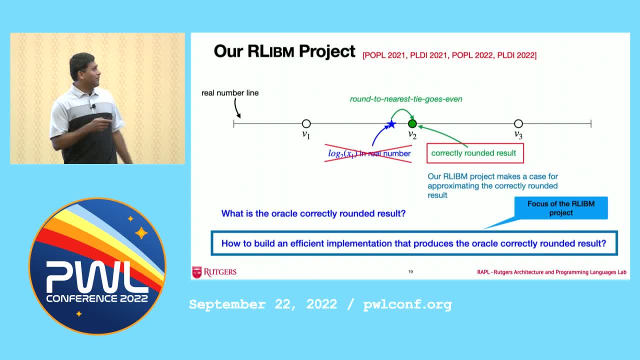 and solve smaller parts and do it well. So we split the problem of generating efficient implementations into two parts: the problem of generating the oracle which tells you what the correctly rounded result is for each input. OK, This can be slow And, like a lot of people, as Zeeshan was alluding to, this is a problem that people have attacked. 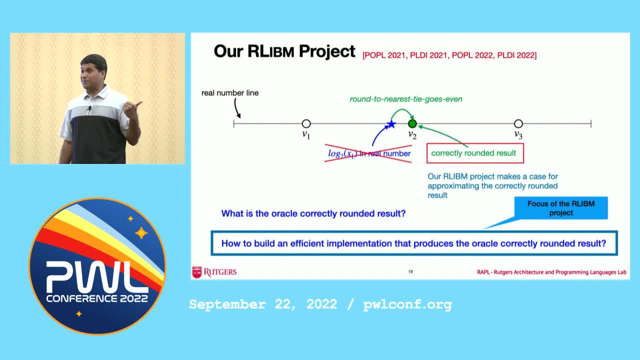 for centuries. OK, So there are good oracles out there, built on the shoulders of giants, Right. So once we know the oracle, what do we want? We want our models to run faster, right. So we want efficient implementation that produce correct result. 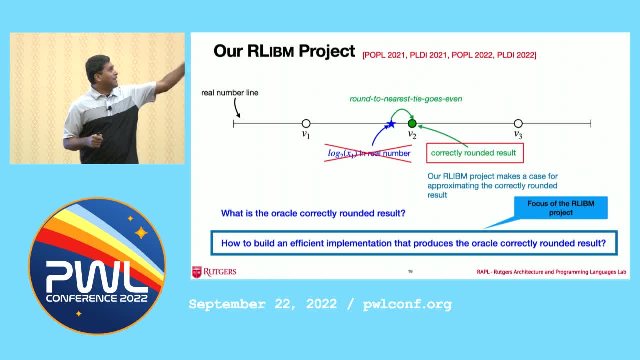 So design efficient implementations by directly approximating the correctly rounded result. OK, The focus of the RLibm project is: given an oracle, let's generate polynomial approximations that produce this result efficiently. OK, So first insight: Directly approximate the correctly rounded result. 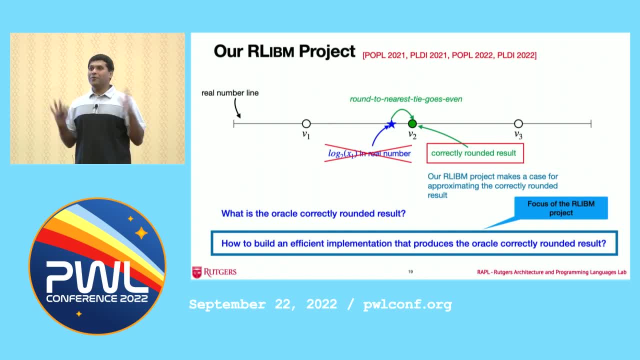 And this is where thinking like a computer scientist actually helps. right, I do have a lot of math background, but to do this, I had to forget some of my math background and think like a person who would implement stuff. OK, So now cool. 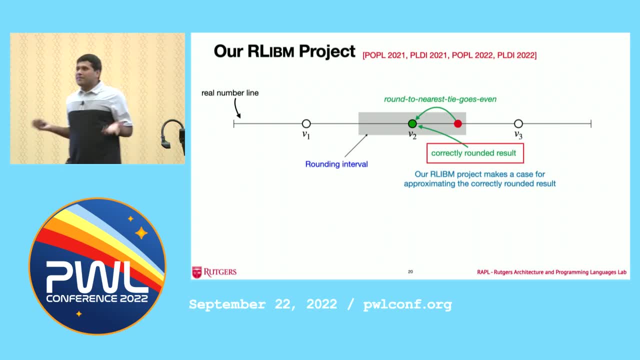 So we want to approximate the correctly rounded result, But that doesn't solve right. But the key insight, the next insight that we had, is, if you have a correctly rounded result, So let's say we are designing a correctly rounded result. So this is a very simple problem. 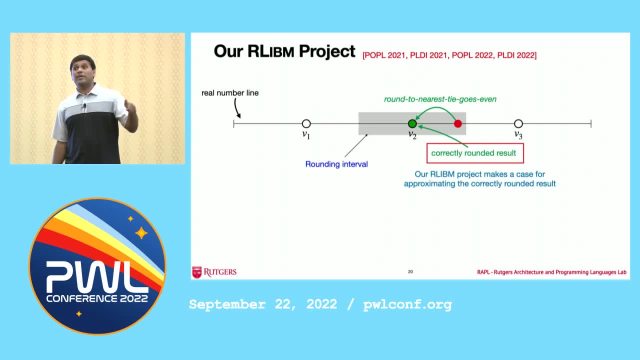 If we were designing a correctly rounded result, we would be designing a correctly rounded result with a 32-bit floating point. How do we where? in which representation do we implement the library? We would implement the library in double precision. So there are a set of real values, there is a range of real values around the correctly. 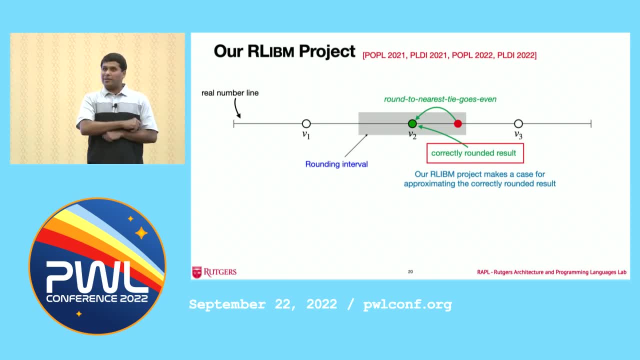 rounded result in the double precision You produce any value there, it will round to the correctly rounded result in the 32-bit flow. This is the freedom that you have. OK, So this gray area is the freedom. So there's a range of values. 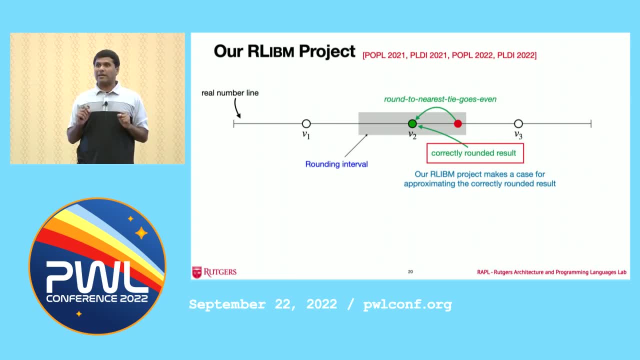 In this case, V1, V2, V3 are three floating point values. V2 is the correctly rounded result. What is the rounding boundary between V1 and V2? The midpoint- And what is the rounding boundary between V2 and V3?? 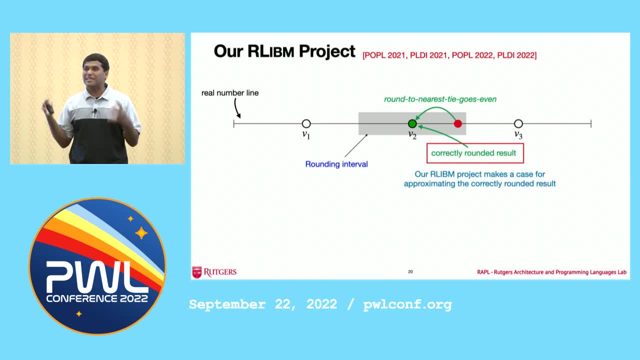 The midpoint. So the region between the two midpoints is the freedom that you have. You produce any real value there. it will round to the correctly rounded result. This is the freedom that our polynomial generator has, And if you recall the figure, this freedom is much larger than whatever you had with 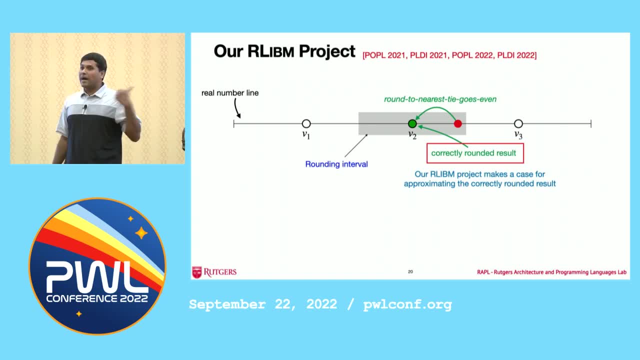 the minimax polynomial And this is precisely why the Arlibm implementations generate really fast implementation Like. more freedom means you can use lower degree polynomials, which implies speed up. So make a directly approximate the correctly rounded result and then there is a range. 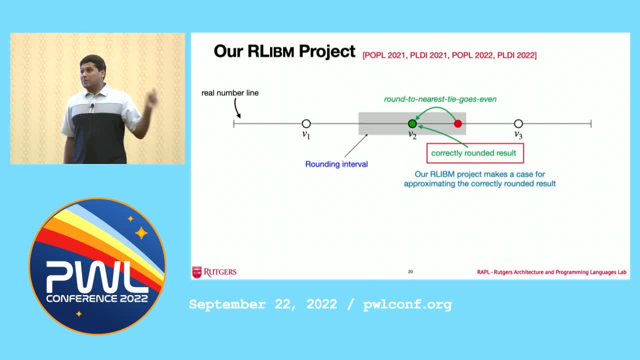 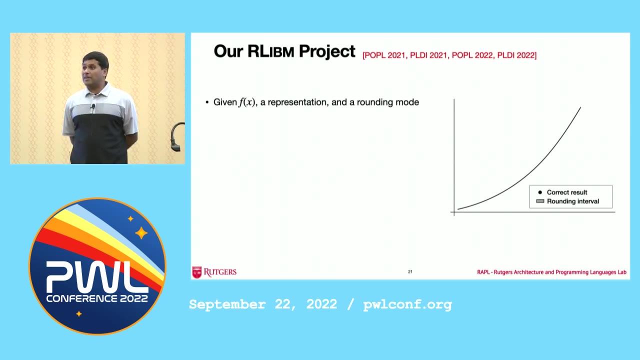 of values around the correctly rounded result, which produces such that if you produce any value in this interval, it produces the correctly rounded result. Now, how do we generate it? The insights are fine. What is the methodology? So our methodology is: we have an oracle, we have the representation and the elementary 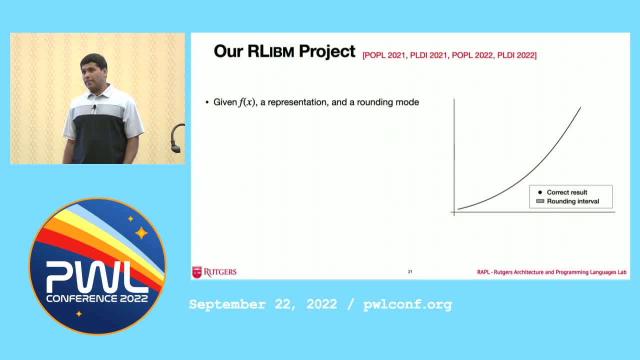 function that we have For each input and a given elementary function and the rounding mode. we would use the oracle and compute the correctly rounded result And then we would compute the rounding interval for the correctly rounded result. And the gray boxes on the figure are the correctly rounded result. 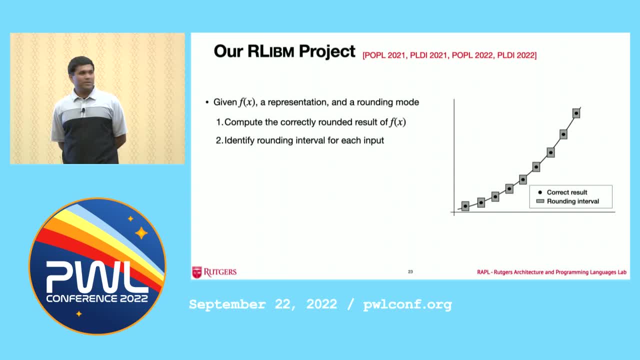 Once you have this, you don't care about the interval. Interval is whatever you care about. Now we want to generate a polynomial that satisfies all these intervals. What is a polynomial? We know the inputs x1, x2, xn- right. 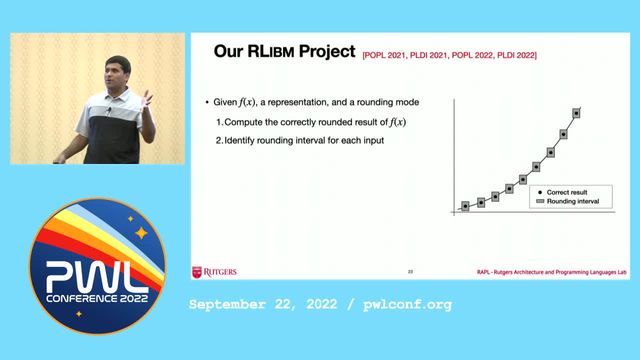 And what we don't know is the coefficients of the polynomials c0 plus c1x plus c2x2.. So the task is to generate these coefficients. So what does each interval specify When you evaluate a particular point? does it generate a polynomial? 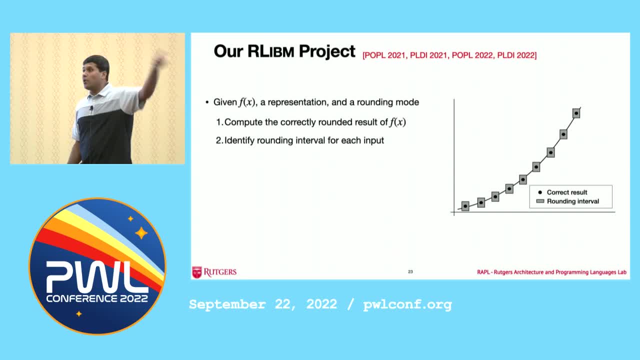 No, The result of the polynomial should be greater than the lower bound and should be less than the upper bound. It's a linear constraint. So, effectively, what do we have? We have a system of linear inequalities for a given degree. Now another well-studied problem: linear programming. 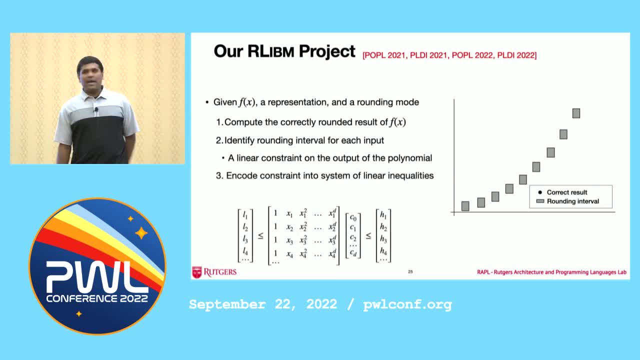 So the very good solvers out there: use an LP solver out there And encode this into a system of linear inequalities. give it to the LP solver. it generates the coefficient. and there you go. You have a polynomial that satisfies all the points. 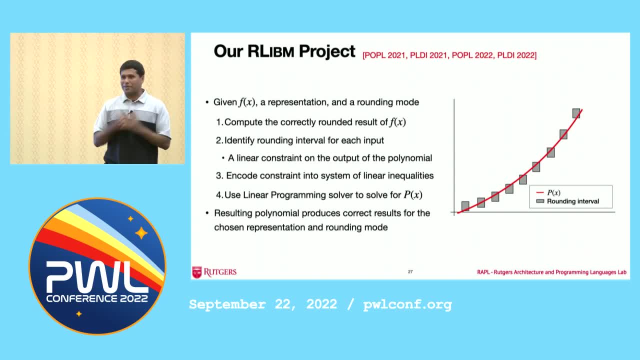 Okay, This is the first insight that we had, like five years, four years ago, And this was our paper where we summarized this result. Okay, What do we have? Directly approximate the correctly rounded result. There is an interval of values around the currently rounded result. then frame an LP. 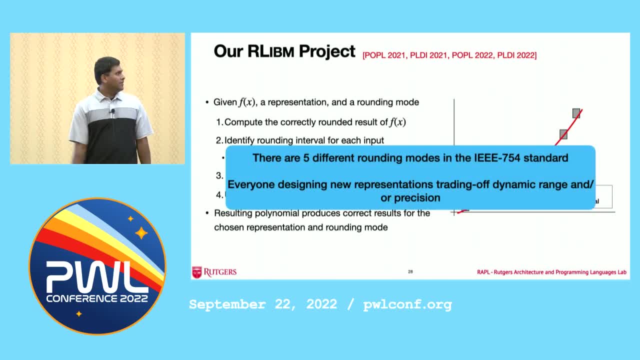 problem and you can generate correctly rounded implementations. So life would have been amazing if there was only one representation and one rounding mode. But today everyone is designing their own representations, trading off the dynamic range or the precision. And if you're still not convinced, just two days ago, a consortium of NVIDIA and Intel 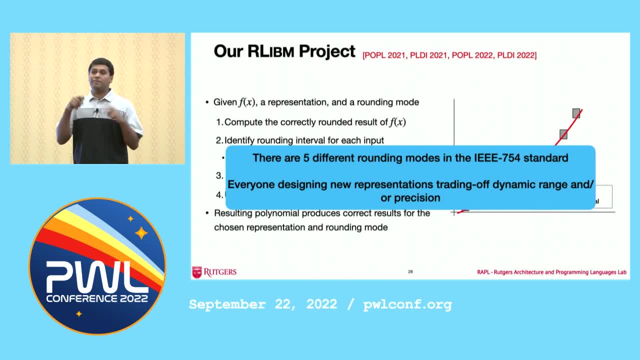 researchers released an archive paper: FP8, 8-bit floating point standard for accelerating machine learning workloads. Okay, It's a cool paper. Look at it like all the tradeoffs that is required to accelerate machine learning. So our next question was: can we design a single representation, a single polynomial? 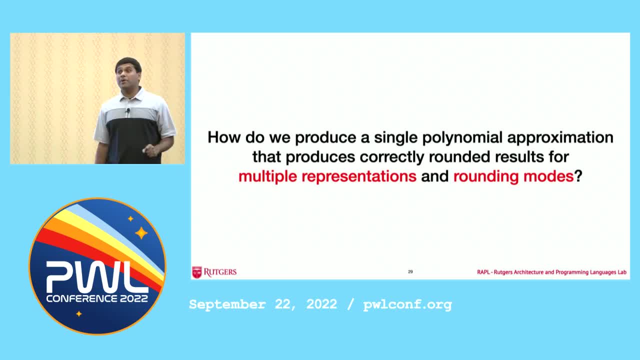 approximation that produces correctly rounded results for multiple representations and multiple rounding nodes. Why is this attractive? You are a library designer. You don't have to design a library for each representation and each rounding. Okay, So then you may be thinking: what is the largest representation that anyone uses? 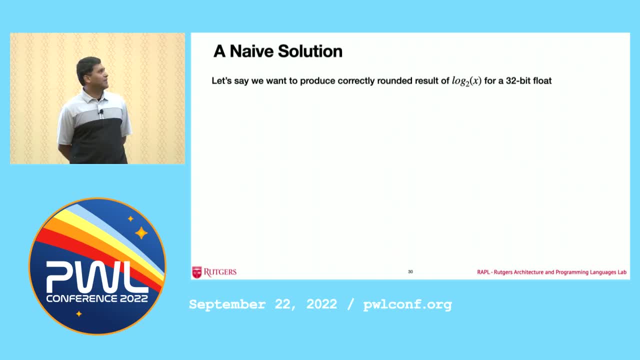 Doubles right Like right now, For practical purposes. Why don't we use a naive solution? If you design it once for 64-bit, are we done? So let's say I designed a correctly rounded library for doubles 64-bit type. 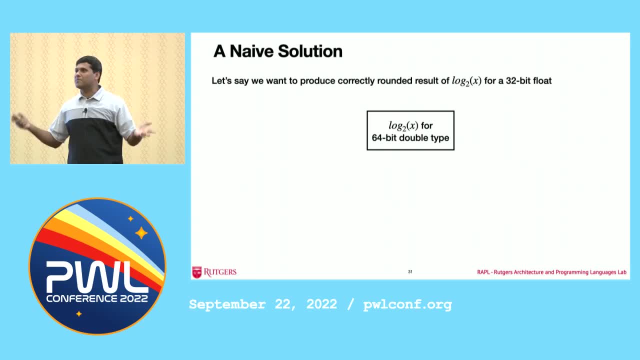 Now what are people doing? Just shrinking precision? Right, I'll just repurpose this library for everything. So what would you do? Let's say you have a 32-bit float, You would create the input. You have an input in 32-bit float. 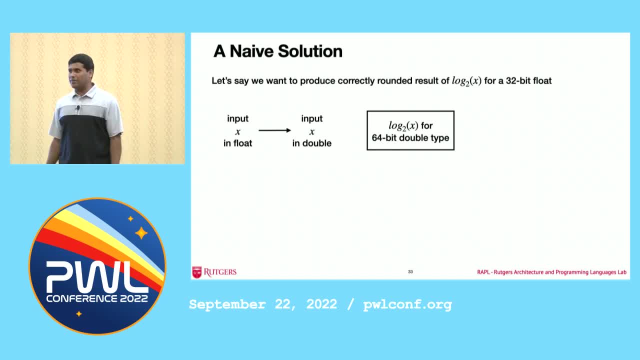 You would promote the input to a double precision. So every floating bit, every 32-bit value, is representable in 64-bit. Okay, And then you call the 64-bit library, You would get the result in, you would get the output in double, and then you would truncate. 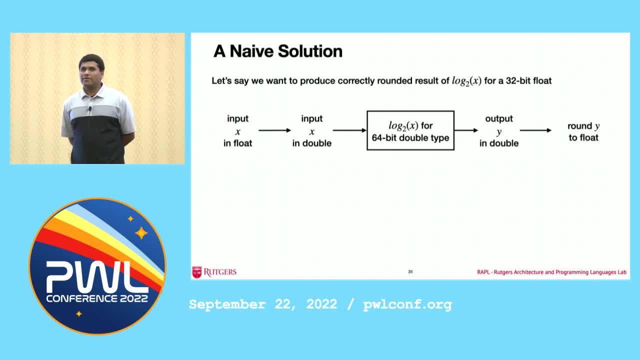 it back to float, round it back to float. Okay, How many of you think like this will produce the correct result? Yeah, Everyone is presuming. I have something to say. This is wrong. This doesn't work. That's a nice solution right there. 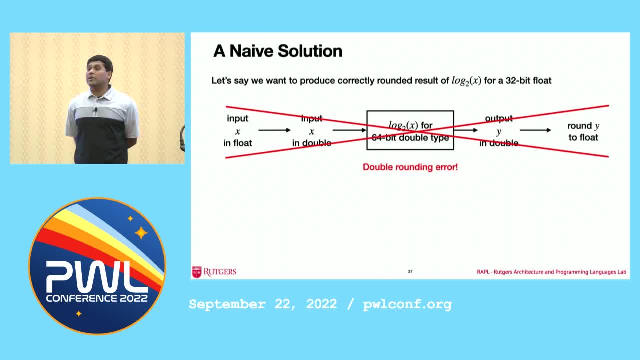 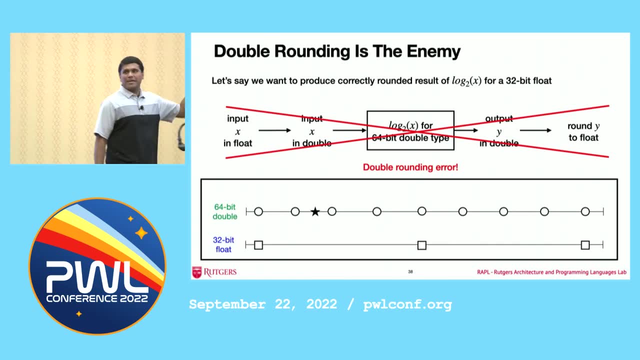 Right. So why doesn't this work? This doesn't work because of double rounding error. What is a double rounding error? So I'm going to demonstrate it here with a cartoonish figure here. So you have 64-bit doubles and you have 32-bit floats. 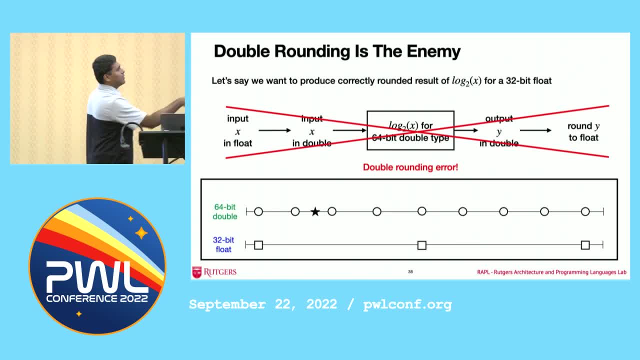 The most important thing is: look at this bottom row. You have a 32-bit float. There are three float values there And there are a lot more 64-bit values between two adjacent 32-bit values. But just for exposition I'm just showing a few values here. 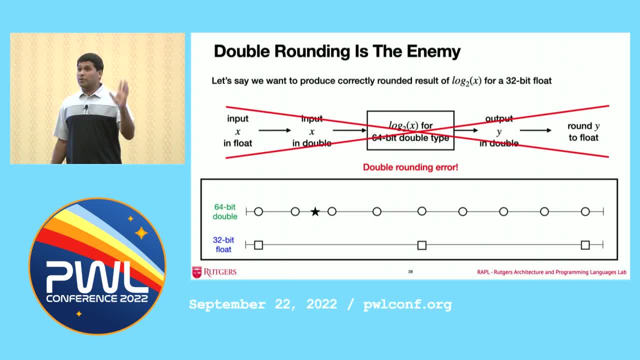 So the star is the real value produced by your elementary function. And now you have a correctly rounded double library. So this is a correct result from the perspective of a double library. Okay, And now, if the value is very close to the midpoint, you round it. 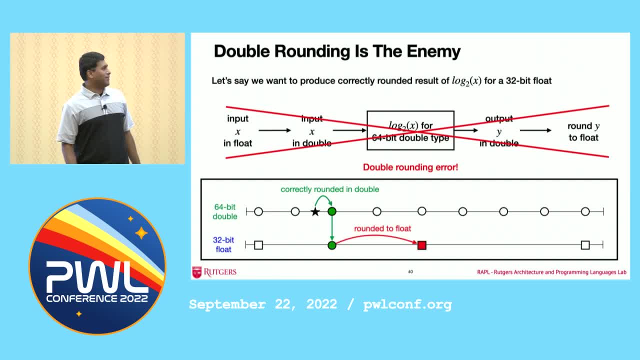 And now, if you take this double value, it's exactly at the midpoint And if you round it to float it produces it rounds to the red box. But if you look at it, this value is less than the midpoint. It should have rounded it to the box on the right. 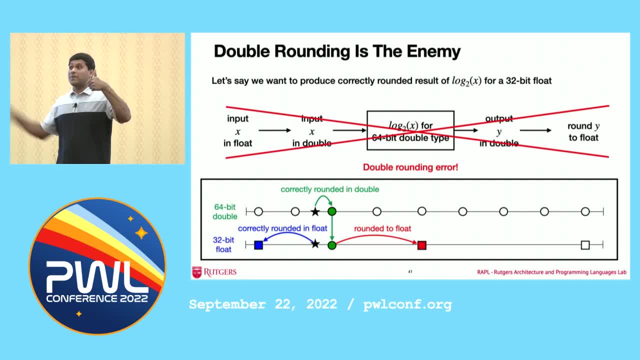 So there are two roundings happening. The first rounding is when the designer of the elementary functions designed it right, Designed the library, So there was one rounding. The second rounding happens when you take the double value and round it to float, And this is very common. 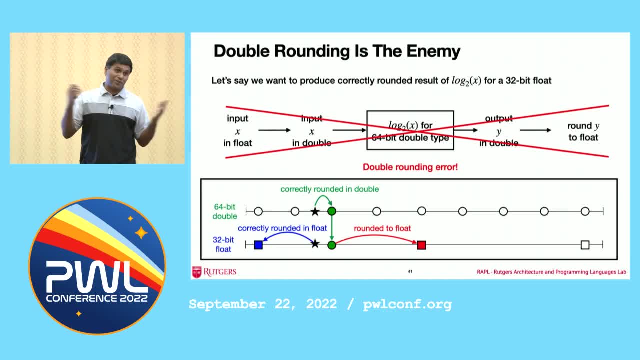 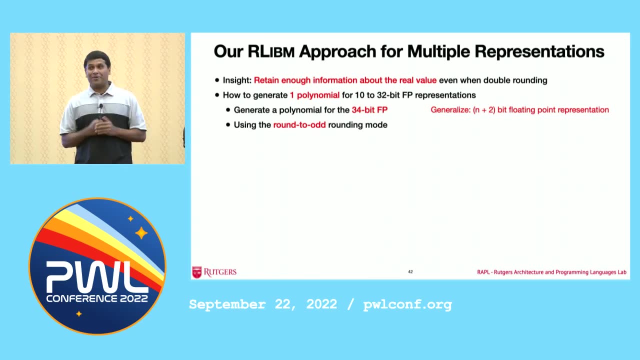 So if you want to generate a single polynomial approximation That works for multiple representations, You need to make double rounding somehow innocuous. Okay, So how do you make double rounding innocuous? So this is our next magical result. This is the advantage of having great students right who come up with really amazing ideas. 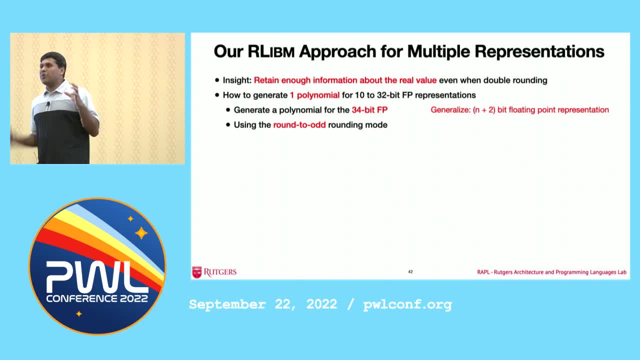 So the real value. like you have to maintain certain information about the real value such that the rounding decision is not changed in the present. So what information do you need to maintain about the real value? So there are three pieces of information that you would want to maintain. 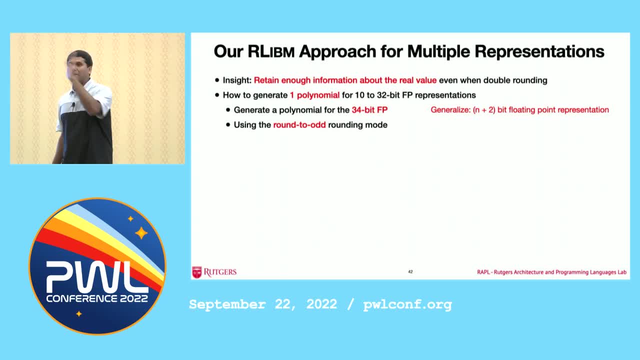 Is the value less than the midpoint? Is the value exactly at the midpoint? Is the value greater than the midpoint with respect to the target represented? If you maintain these three pieces of information exactly, you can make double rounding innocuous. Okay, So this is the key insight. 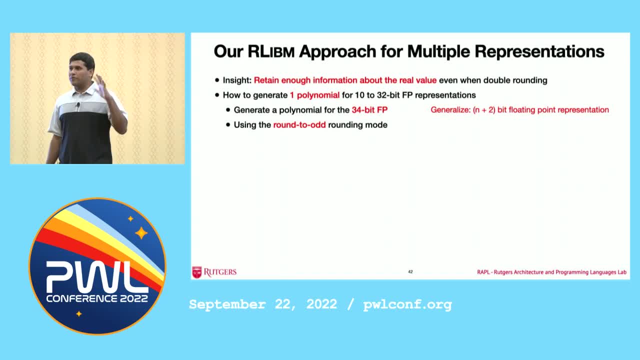 But what is our magical solution to address it? Okay, So if you want to create a correctly rounded library for all representations up to n bits, okay, create a polynomial approximation, a correctly rounded polynomial approximation for n plus two bits, two additional bits with a nonstanding rounding mode called round. 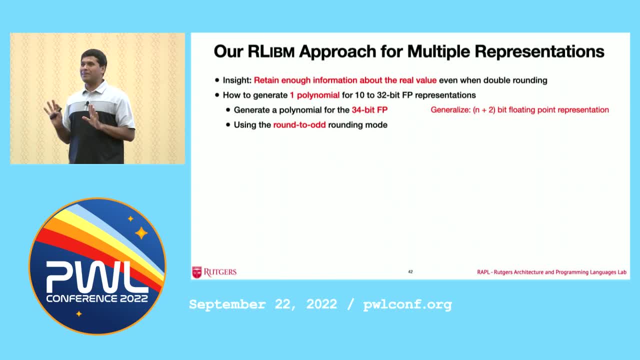 to odd And I'll describe what round to odd in a minute. And if you magically double cast this, double round this to any representation from one to 32 bits, it will produce correct results And all the five rounding modes in the standard. 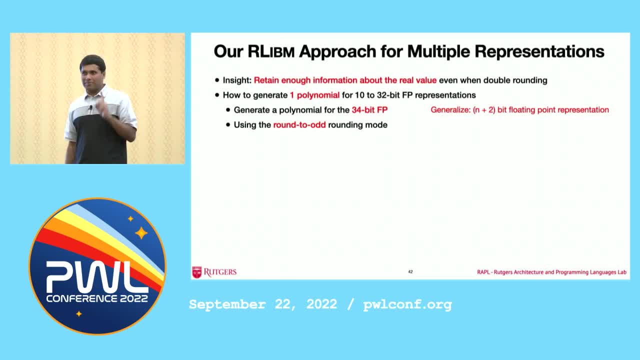 Okay, So now there are a lot of things to pass. The first thing to remember is, if you want to generate correctly rounded results up to n bits, create a library with two additional bits with a round to odd mode. Now, what is a round to odd mode? 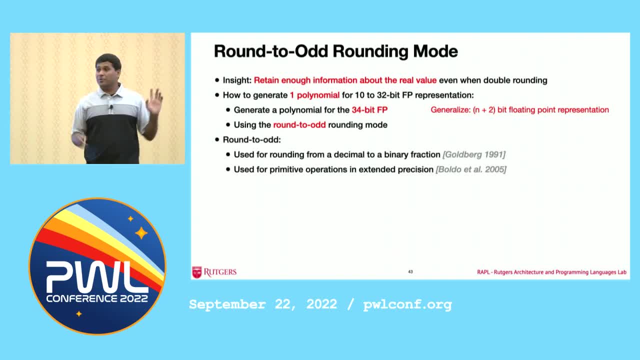 Okay, It's a nonstandard mode. People have looked at it Like if you read a paper titled Walt, Every Computer Scientist Needs to Know About Floating Point by Goldberg Right. So there is like he references to it. Okay, When he's talking about casting, converting a binary fraction to a decimal fraction. 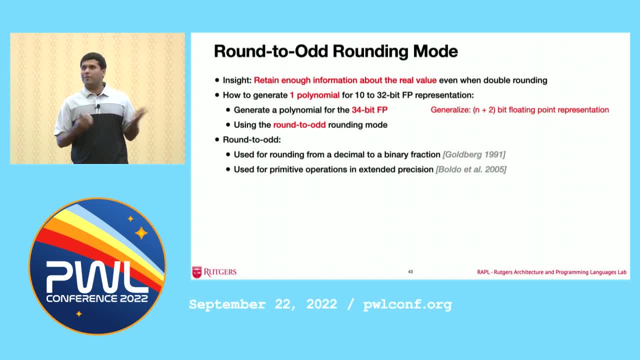 And why haven't people used this round to odd mode for elementary functions? Because people have been obsessed about real values. They've never been thinking about specific rounding modes for generating libraries. So, in contrast, in the ArlibM project, since we directly approximate the correctly rounded 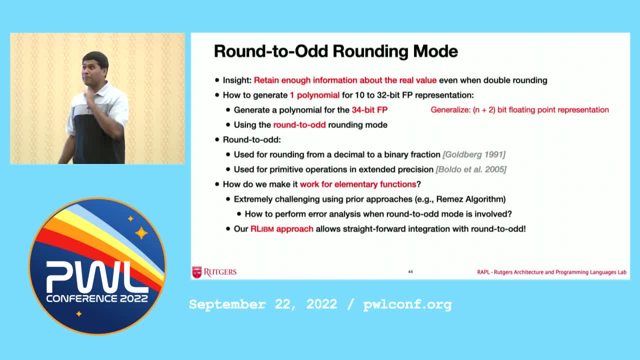 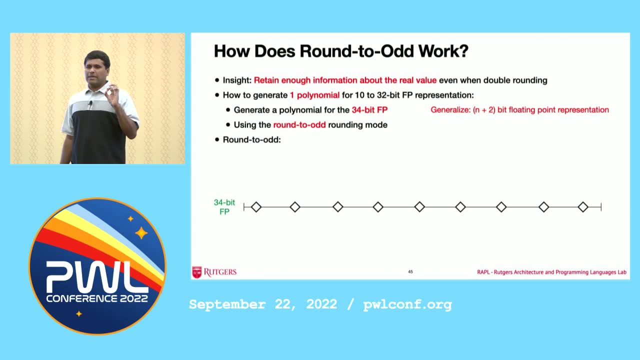 result we can generate directly, approximate the round to odd result And still be, we don't need any additional numerical analysis. So now let's walk through the intuition. So what is round to odd? So round to odd mode is explained in two sentences. 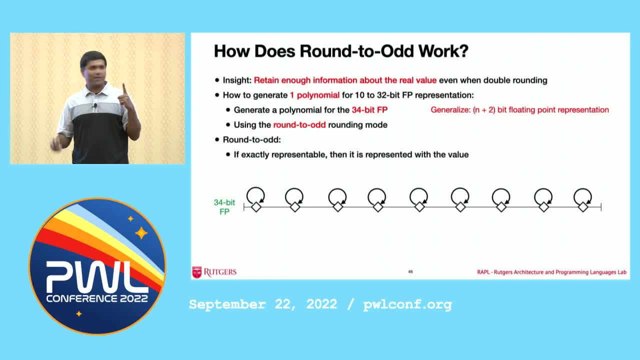 First, if the value is exactly representable, it rounds to this value. Okay, So if the value is exactly representable, it rounds to that value. If the value is not exactly representable, then it rounds to an adjacent value. Okay. 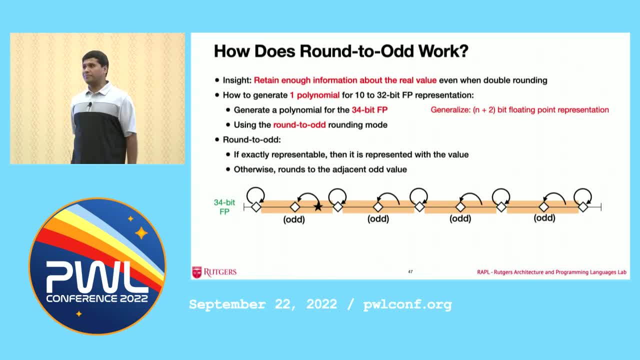 So if the value is not exactly representable, then it rounds to an adjacent value. Okay, So what happened is that our bit pattern is odd. Okay, So there are a lot of things in the slide, but let's go back and step back and give. 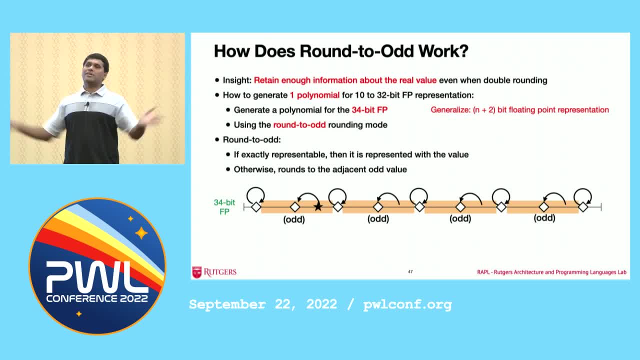 you a very pedantic example. Let's say we live in a world where we just have integers, Okay, And you produce a value 9.6.. We just have integers, You produce a value 9.6.. You need to round. 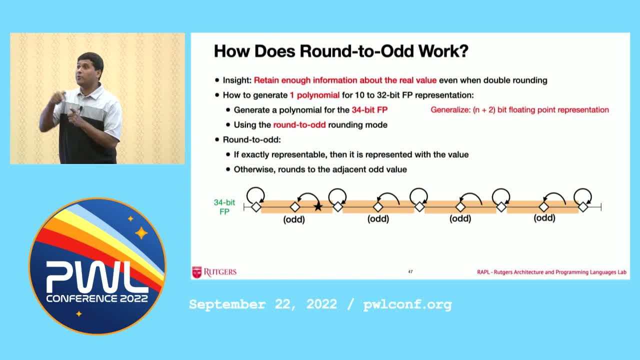 Now, 9.6 is not exactly representable as an integer, So you need to round. Where do you round to? In your typical, usual world, you would round to 10, with round to nearest. With round to odd, you would round to 9, because 9 is odd. 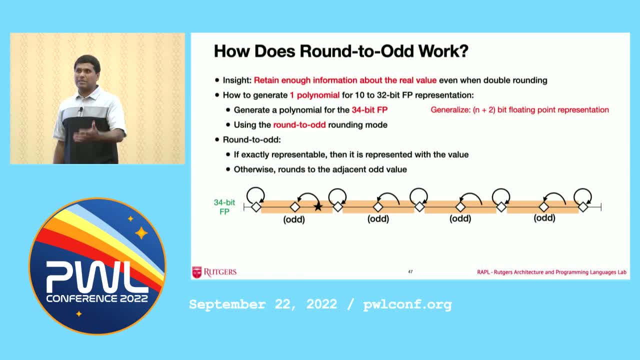 So this is round to odd mode. So just to reinforce this, let's say you have a value 10.3.. 10.3 is not exactly representable, so you would round to 11, because 11 is odd. So the round to odd if the value is exactly representable. 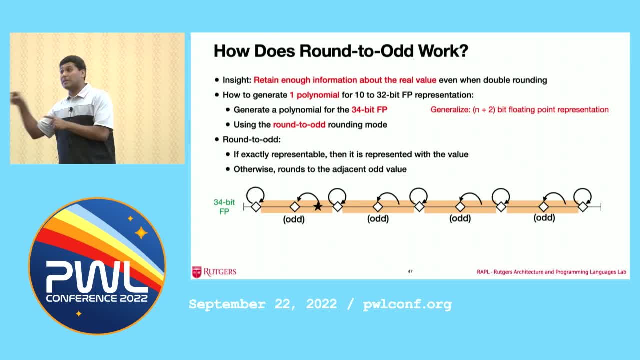 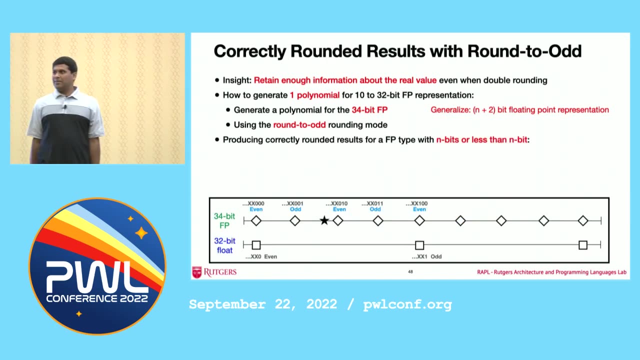 it rounds to that value. If it's not exactly representable, it rounds to a nearest value because the bit pattern is odd. So this is round to odd. Now, round to odd makes double rounding innocuous. Why So? let me illustrate this. 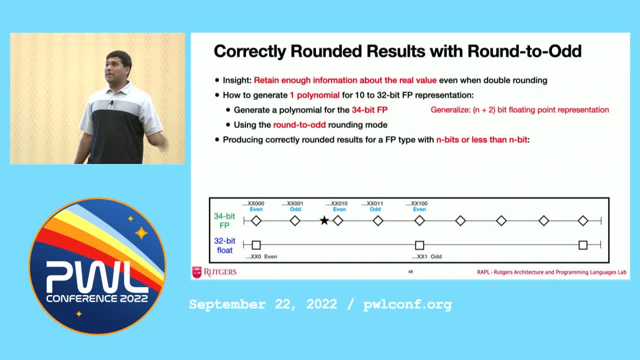 So let's say we are designing a correctly rounded library that produces correct results for all representations up to 32 bits. So then we need to create a polynomial approximation for a 34-bit library. So here in the second row, I'm showing the 32-bit values. 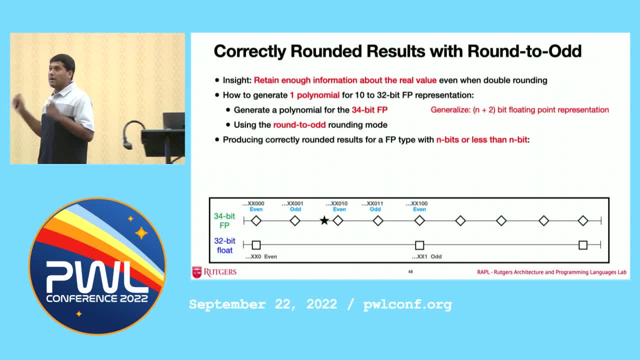 And in the first row I'm showing the 34-bit values. Between two adjacent 32-bit values, there are three 34-bit values exactly representable. So now, irrespective of whether this bit pattern is even or odd, any value that is representable in 34 bits. 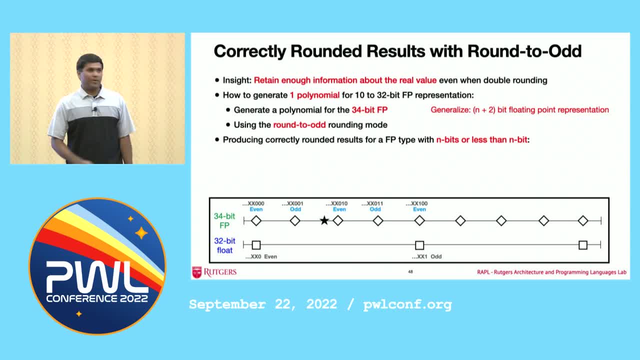 will be even in a 34-bit representation. OK, So this will be even. This will be odd. This will be even. This will be odd. This will be even in a 34-bit representation. So now the key point to remember is: what are the key things? 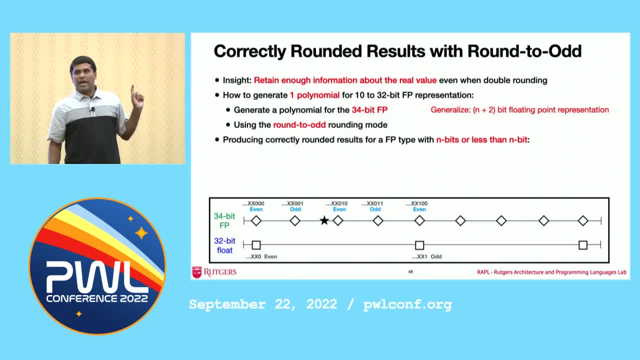 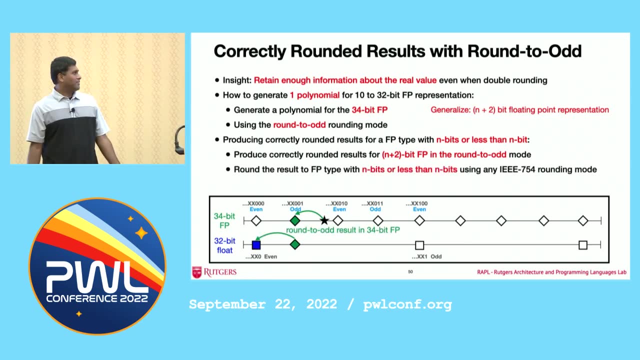 The midpoint is even in 34-bit And any value less than the midpoint, any value less than the midpoint, it rounds to the odd value with round to odd. So it rounds to this green value. OK, So now, if you double round it later on, 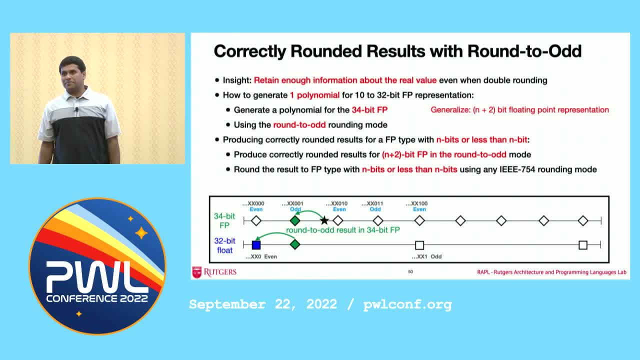 it will round to the correct floating point result. OK, So the round to odd preserves this information, the three pieces of information that is required to correctly round any values. What are those? Is the value less than the midpoint? Is it exactly at the midpoint? 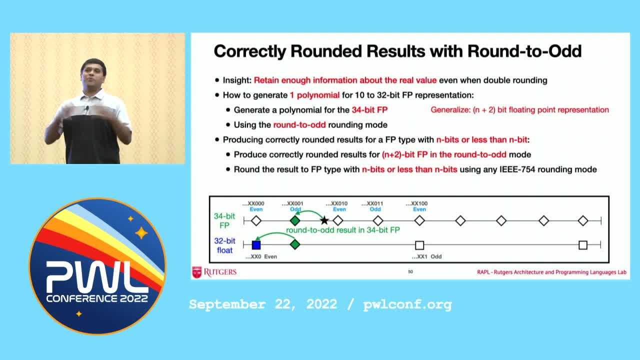 Is it greater than the midpoint? So the proof is a bit more involved. I don't want to burden you with the details of the proof, But the key theorem that we prove in the paper OK Is: take a real value to round a real value. 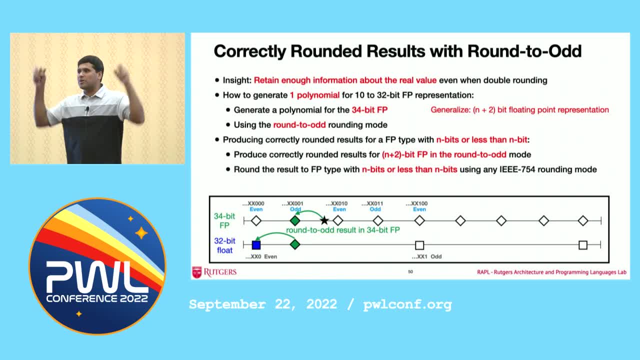 to any representation. there are four pieces of information that you need, which we call as the rounding components, And what we show is the round to odd mode preserves the exact same rounding components for rounding any real value to any representation. OK, So the end result is: if you want a polynomial, 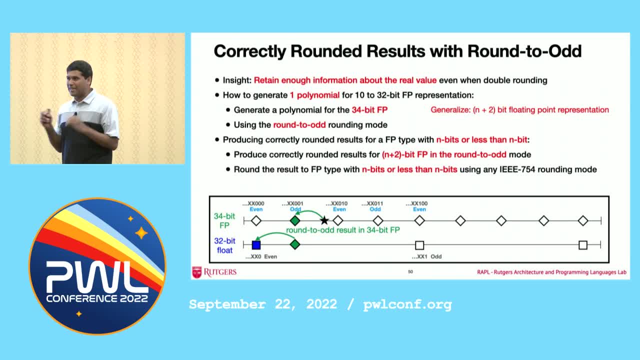 if you want an approximation that produces correct results up to n bits, create a library That produces correct results for n plus 2 bits with a round to odd mode, And it magically produces correct results for all representations and all five rounding modes. So now the question is: how do we go about creating this library? right? 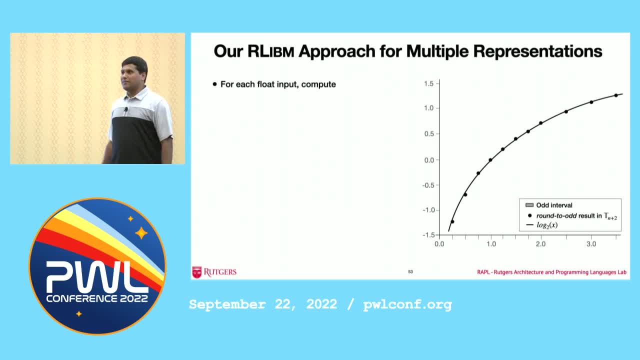 So we exactly use the Arlibem approach. So you have an oracle. In this case there is no oracle which gives you 34-bit. We build the oracle for producing 34-bit round to odd mode. For each input we would compute the correctly rounded round to odd result. 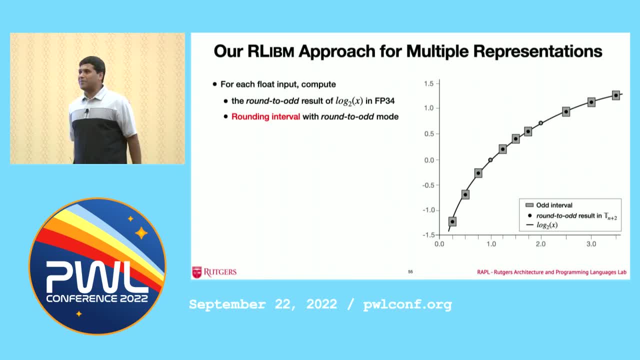 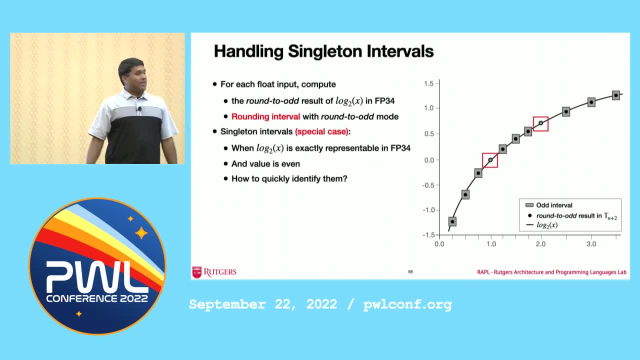 OK, And then we generate the rounding interval, so the odd interval, so that every value rounds to the correctly rounded odd result. And then the only issue that you need to worry about here is if the value, if the result of an elementary function. 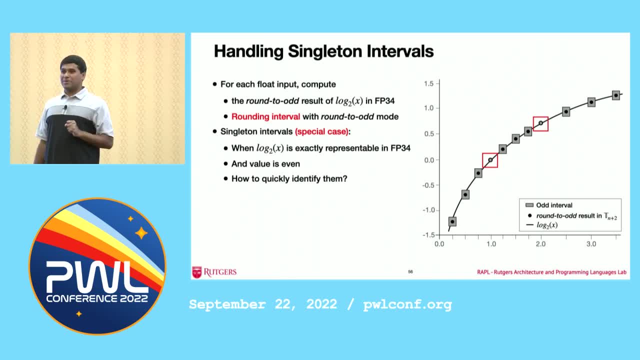 is exactly representable in your representation and is even it's odd interval, is a singleton. generating singletons is challenging, But fortunately this problem of identifying singletons in the context of elementary functions is well-studied. So what is a floating point input? 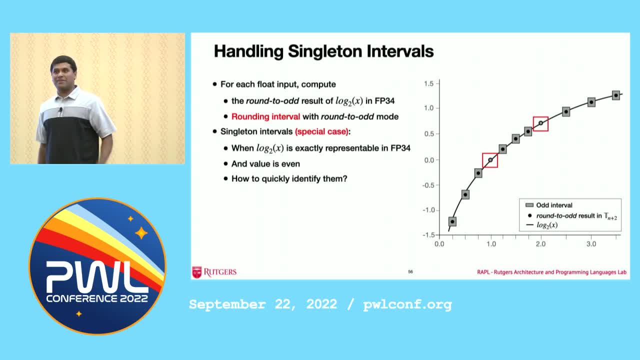 It's a rational value. If it's exactly representable in a floating point representation, it means it's a rational output. So what we are looking for is you have an elementary function which takes rational inputs and produces rational outputs, And there are some fantastic results. 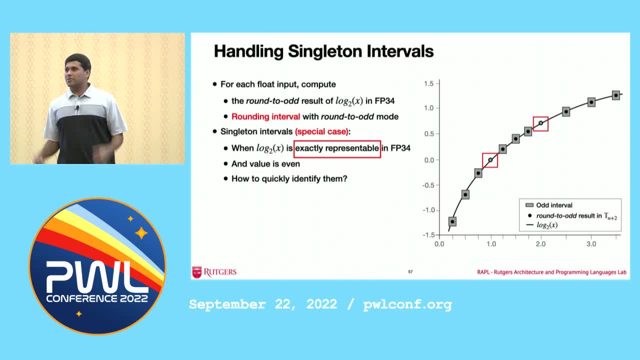 OK, OK. So let's take a look at the real analysis which we use. So just to give you an example, let's say we are computing log x to base 2.. So when i is an integer and even then log x to base 2, 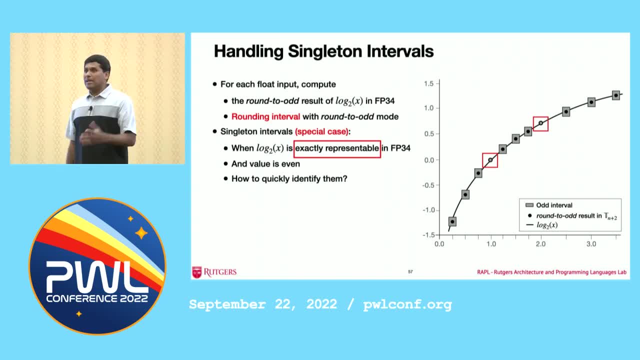 is exactly representable and it's even So. it will be a singleton. So we use bit vector operations to compute such results and remove the such singletons. OK, So once we remove those singletons, we are left with odd intervals. 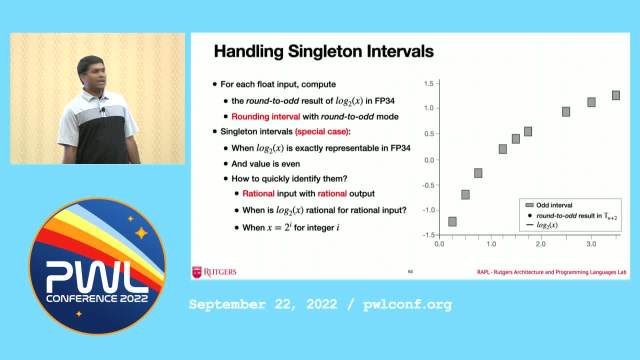 We generate a polynomial for them And it produces correct results for all inputs. OK, So what are the three takeaways I want till now? There's one more takeaway, but three takeaways till now Directly approximate the correctly-rounded result. 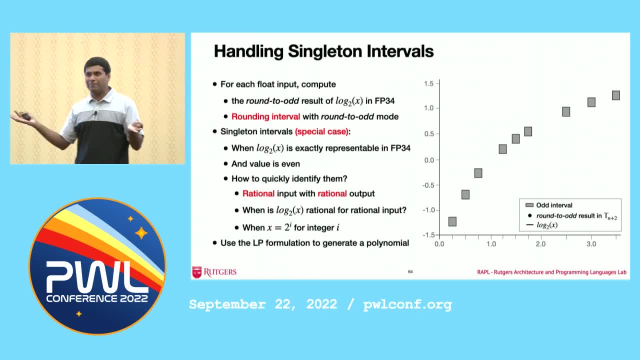 Then there is an interval of real values around the correctly-rounded result Frame- an LP problem. And if you want a single polynomial that works for multiple representations and rounding modes, create a polynomial approximation for two additional bits, n plus 2 bits with a round-to-odd mode. 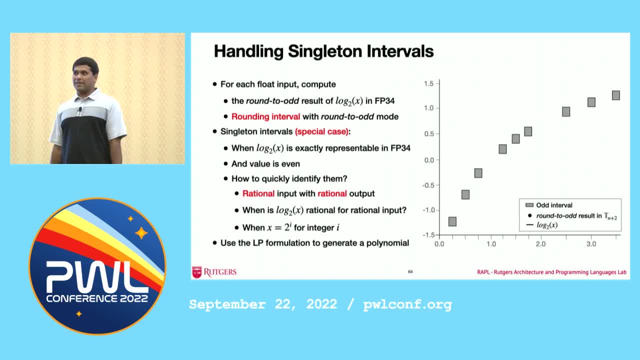 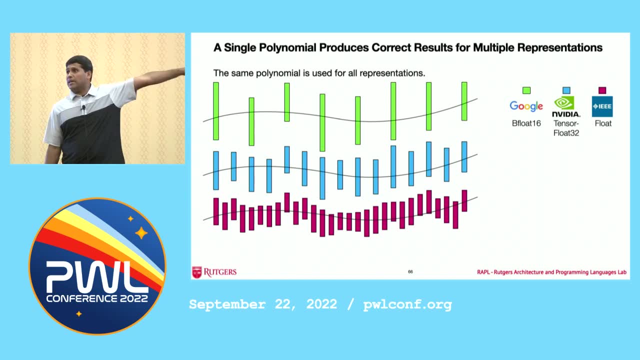 and it magically works OK. So the last thing that I have been talking about is how do we generate this, how to solve this LP problem. So what do we have? We have a single polynomial that works for all representations And if I generate it for 32-bit float, 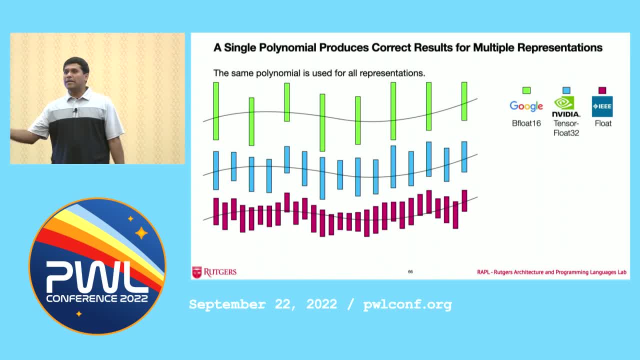 it includes the 16-bit float, bfloat16 from Google, NVIDIA's 19-bit tensor float 32 representation, half-precision, and all other representations, many other representations that people are worried about. So one of the questions I got when I gave this talk a year ago: 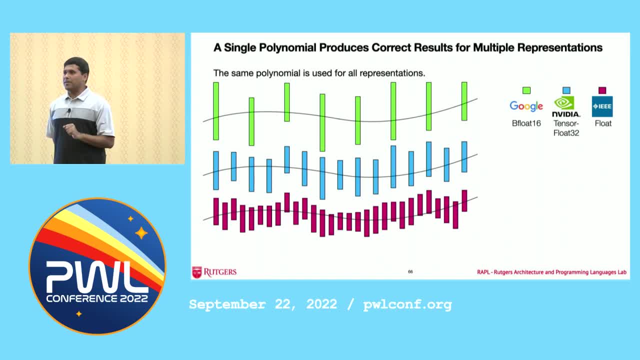 was. this is all great, It's amazingly good, But you're making my bfloat16 library pay the cost of 32-bit float. Can you make it better Again? this is why you meet people and get feedback. They ask questions and I think 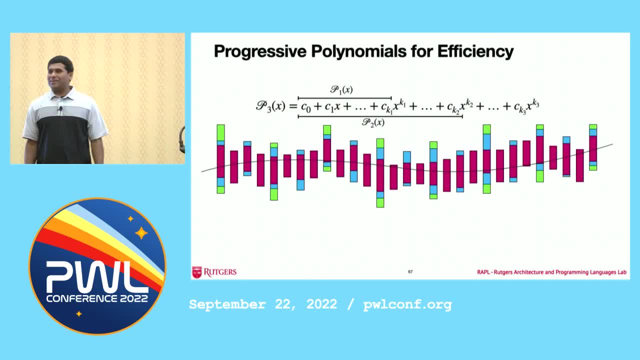 So can we do better? OK, And this is where we introduce this notion of progressive polynomials. So you have a single polynomial that produces correct results, with a round-towered mode for all inputs and multiple representations, If you care about a couple of representations. 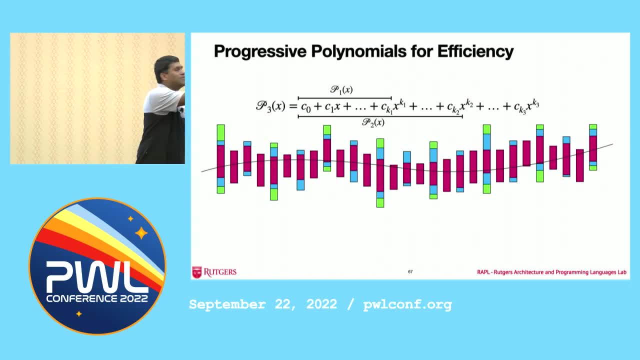 let's say bfloat16 and tensor float32, you just use the first few terms of the same polynomial: It produces correct results for bfloat16.. And additional few terms: it produces correct results for tensor float32.. So in our formulation, how do you do this? 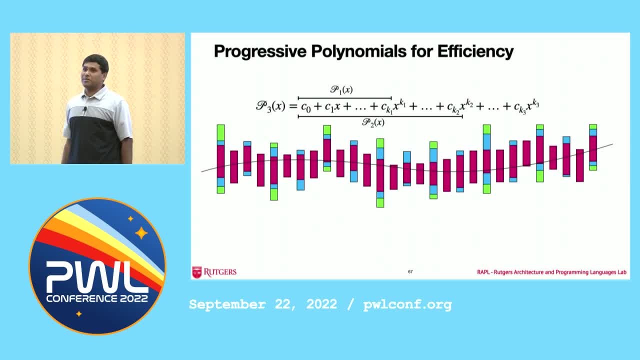 You just discard the higher order terms when we generate the constraints, So it just results in more constraints in the LP formulation. So the entire polynomial produces correct results with a round-towered mode. And then, if you just want correct results for bfloat16,. 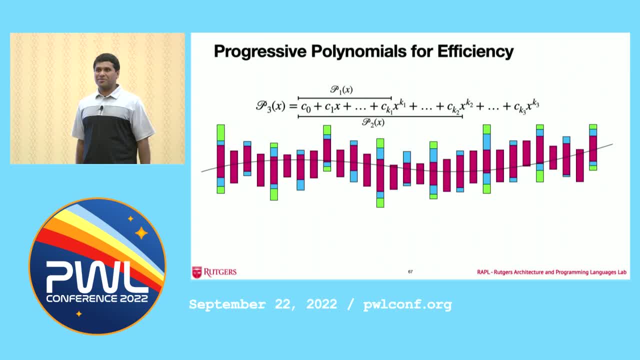 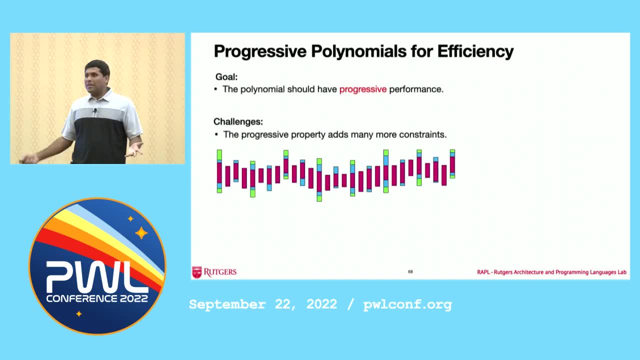 you just don't include those terms in your constraint generation. So there is such a polynomial which has this property. It's a progressive polynomial. OK, so the only challenge now is: do I want it to be bfloat16?? is you have more constraints With 4 billion inputs? you already have 4 billion constraints. 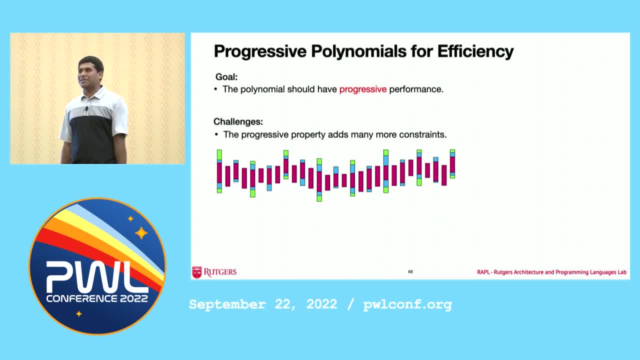 Now, on top of it, you added additional constraints for B Float 16 and TensorFlow 32.. Now we want to solve an LP problem with 4 billion constraints. How do we do this? So we are relying on LP solvers to solve them, Even though LP problems have been well engineered. 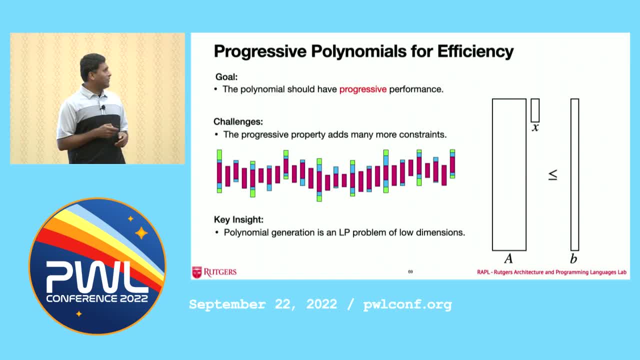 they can't solve 4 billion constraints. They time out. So we had to be clever. So the first observation that we do is our LP problem. the linear program that we generate is a linear program of small dimensions, Even though we have 4 billion constraints. how many terms? 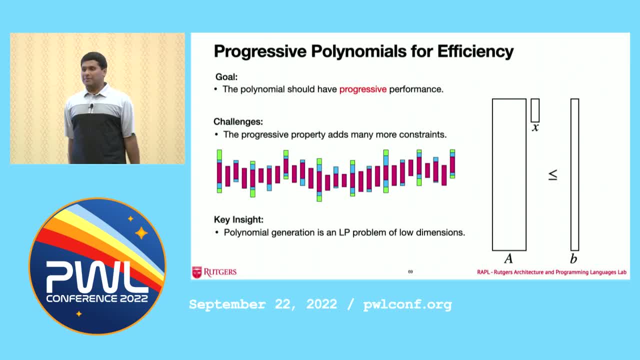 do we have in the polynomial? Very small. We are not looking for 1 billion degree polynomial, We are looking for a polynomial of degree 5 or 6. So the number of terms are pretty small. So our linear program is a linear program of small dimensions. 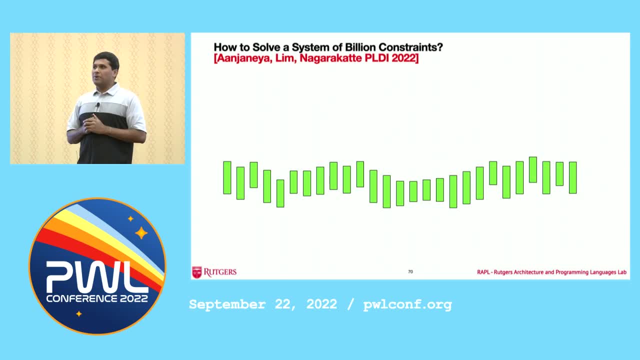 So we have an efficient algorithm to solve that. So we have a linear program of small dimensions. So we have an efficient algorithm to solve that. So what is the key idea? So if your linear program is full rank, that means there are K constraints that satisfy. 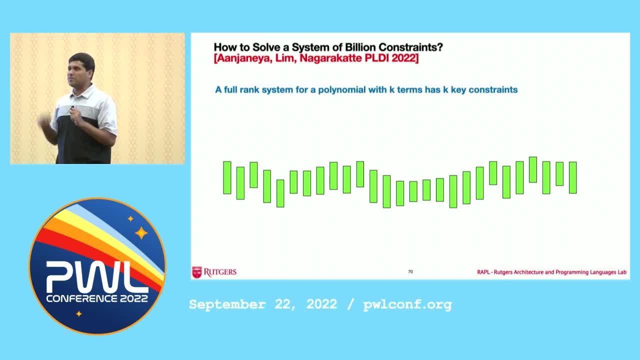 all other constraints There exists, like K, critical constraints. If you just identify them, it will solve the entire problem. So now, how do you identify these K constraints from 4 billion constraints? This is where we employ a randomized algorithm inspired by a classic result from 95, from 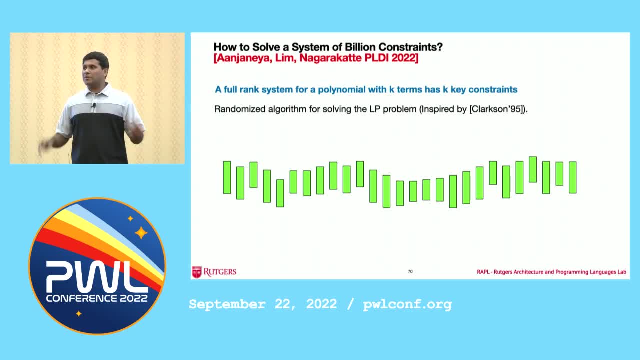 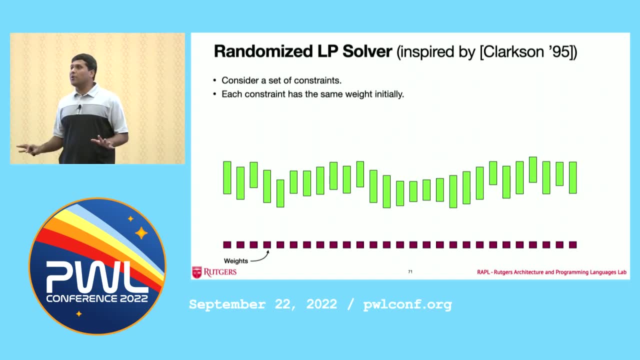 Journal of the ACM Clarkson's method. So I'll give you the sketch of the randomized algorithm. So we have all these 4 billion constraints And we are going to do sampling, we are going to assign weights to each of these constraints. So initially, all these constraints have weight 1.. 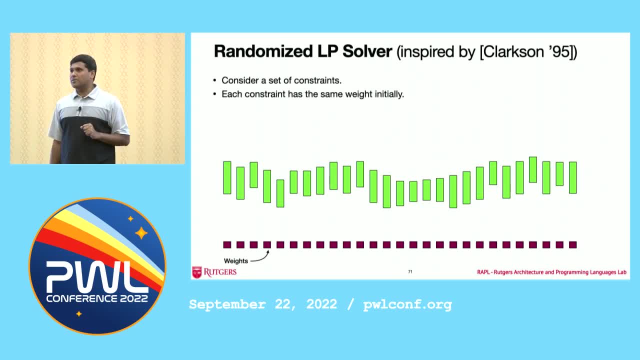 So the first step is just uniformly sampling some constraints. How many constraints do we sample If the polynomial has K terms? we sample 6 K squared constraints. So it's degree 6, let's say the 6 terms 6 times 25, which is 150 constraints. 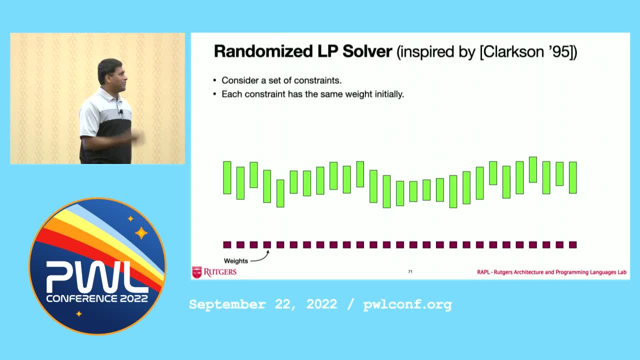 And any LP solver can solve it. So we are in the realm of modern LP solvers, So we sample these constraints and generate a polynomial. So the sample is satisfied by the generated polynomial And it may not satisfy many other constraints in your universe. 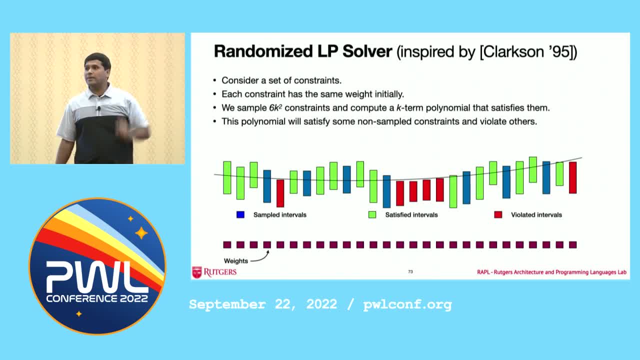 So we evaluate and test it out And it turns out all the red constraints have not satisfied. So we double their weights. What is the goal? In the next sampling we should increase the probability of picking them. So we do weighted random sampling. 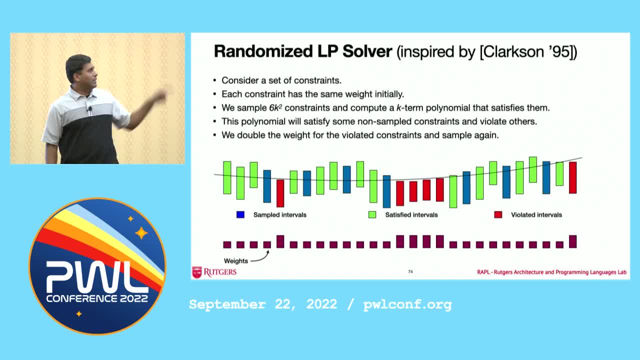 So now we discard the sample and repeat the process. So now we double the weights and we re-sample again. Now some of the constraints, which was weights were double, will now be in the sample. So we repeat the process And check. 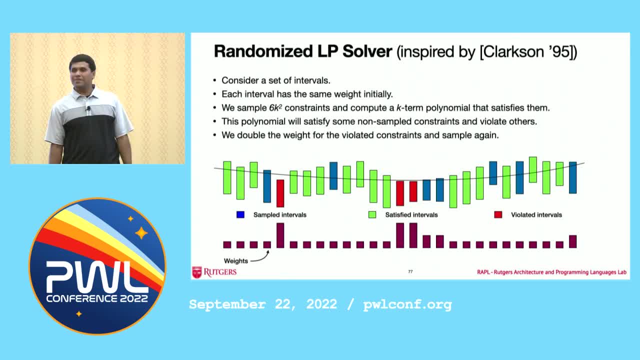 They violate some other points, Now double their weights again And in the next sample, when we do weighted random sampling, we pick a new sample And repeat this process. Eventually you end up with K constraints in your sample And it satisfies the entire universe. 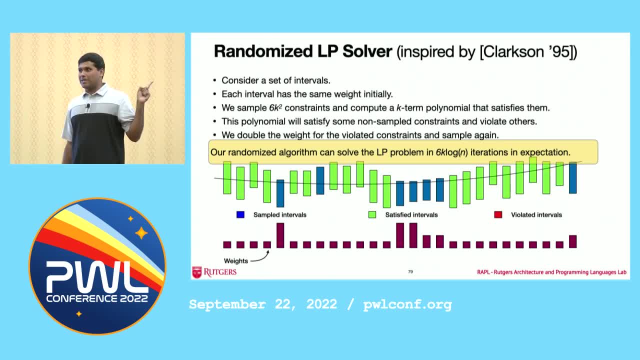 So in our paper we provide the proof that this randomized algorithm terminates in 6 K log n iterations in expectation. So this is a worst-case bar. OK. So randomized algorithms. So designing a randomized algorithm is easy, right, Providing the bounds is the hard part. 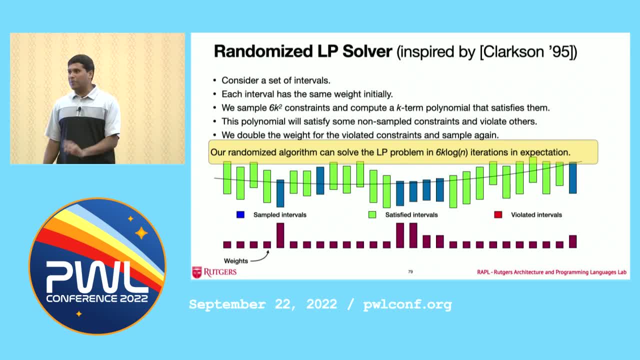 So the proof is a bit involved, But it's easy. Still, it's easily doable. So the end story: In practice. we see this much more effectively. We don't need all these iterations. This is a worst-case bar. 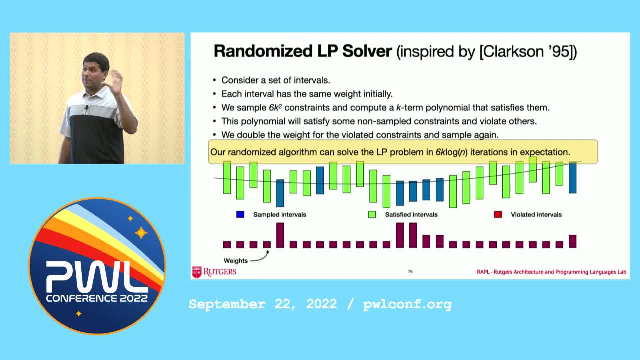 So what do we have Now? we know how to generate like insights behind generating correctly-rounded libraries. We know how to solve the problems effectively, And this is all nice stories that I have been telling you for the last 30 minutes. I hope you enjoyed it. 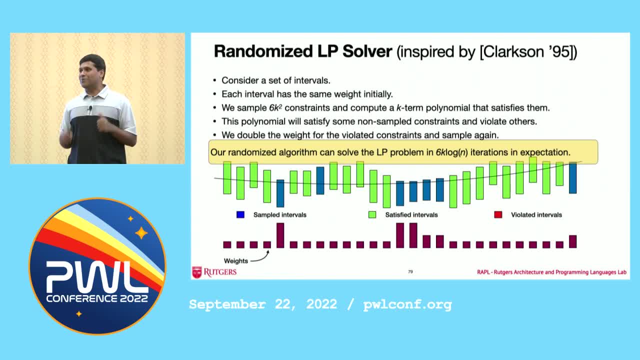 Thank you. That's just a 3-minute story. You can keep on talking for 40, 50 minutes. At the end of the day, what do you care about? Does it work? OK? So we built a collection of ten functions on this slide. 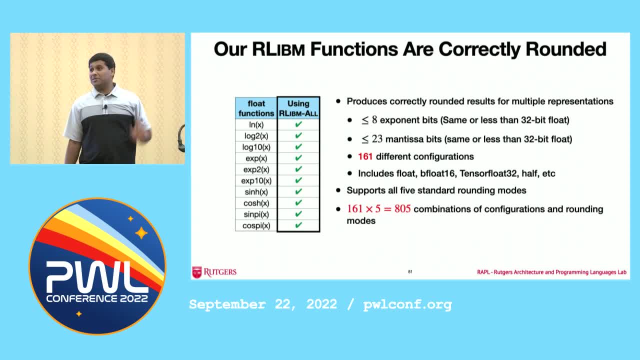 But this is like paper, soo-y love, right? I am just presenting the four papers as part of it, But like the project has like 19 functions, including all the trigonometric functions right now. So single polynomial produces correct results for 805 different configurations. OK, and 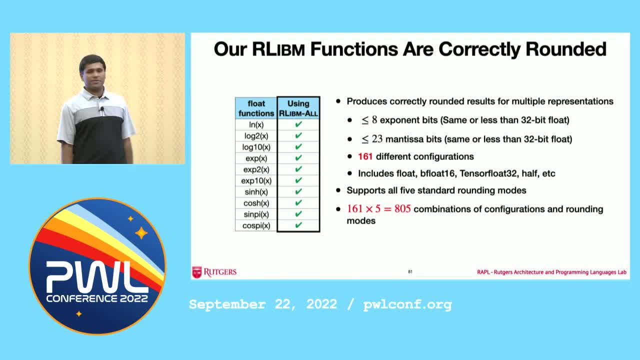 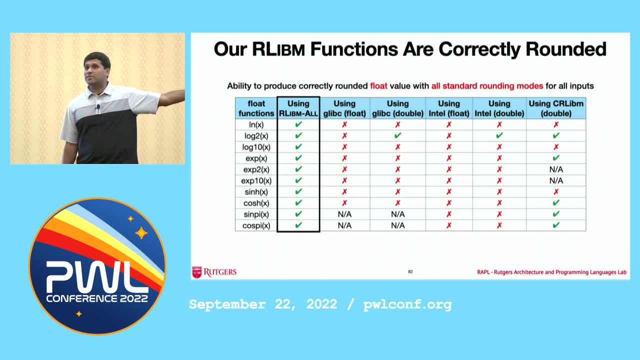 for all inputs: 2 power, 32 inputs. All right. All right with the floating point representations, And just to give you a flair for how others fail, these are like libraries that have been optimized for decades, so not just a couple of years, right. 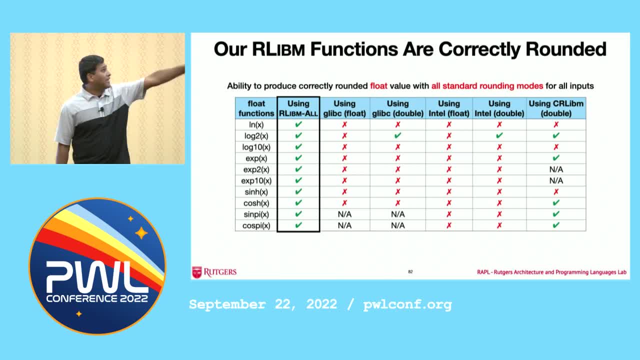 Like they produce wrong results. okay, And even correctly rounded, it's a correctly rounded library developed at India. It's a correctly rounded double precision library. But because of double rounding error, if you take that result and round it to any other representation, it produces wrong results. 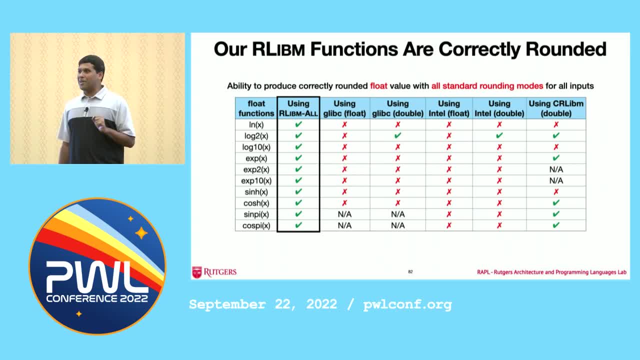 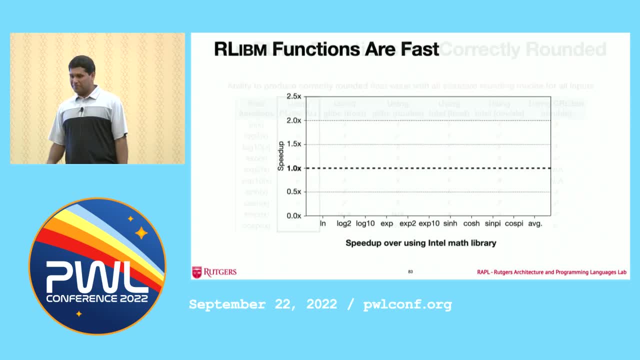 It does not produce wrong results. So the moral of the story is: rlibm functions are correct, So now the next question is: what are we paying in terms of performance, right? So now, in this slide, I'm going to show you what is the performance speedup with rlibm. 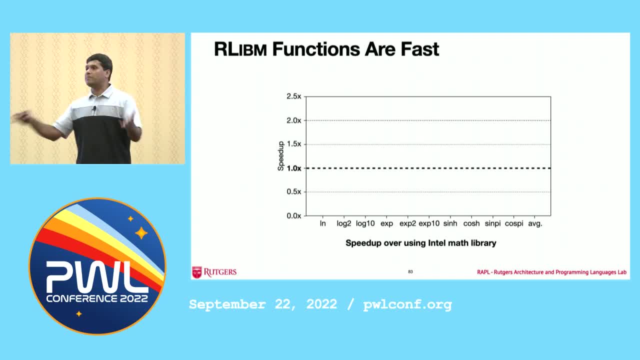 functions. So the line at one means we are as good as the baseline library. So the baseline library is Intel math library, Very well optimized, Like amazingly respected people. So Intel library has two modes. One: you can approximate float functions using float itself. 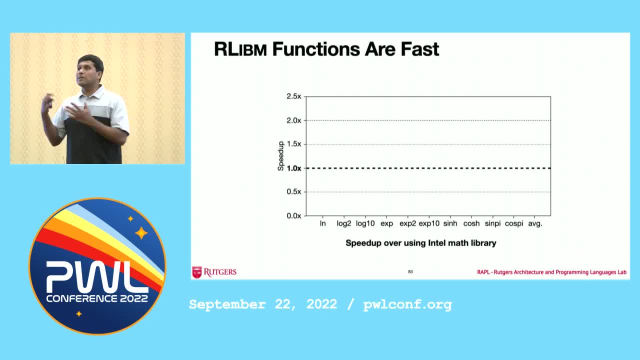 And you can approximate float using double precision. okay, So the approximating float functions using double precision reduces the number of wrong results, But still not correct for all inputs, but reduces the number of wrong results. okay, So compared to Intel's float functions, we are about 30% faster on average. 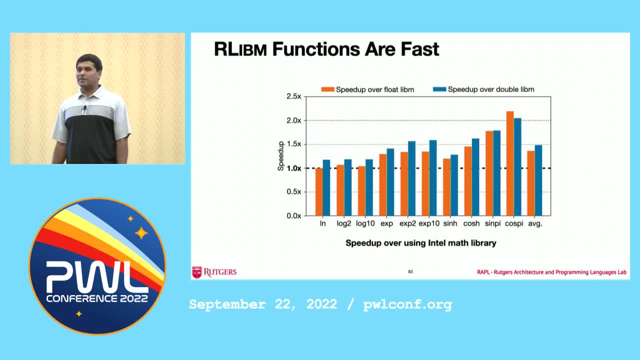 And when you look at double functions, We are about 50% faster. And these slides are like one year old now Because, like all the papers, we are talking about published papers, right, So there's a lag of one year. If you go and download my GitHub library and test it out, your results will be more like: 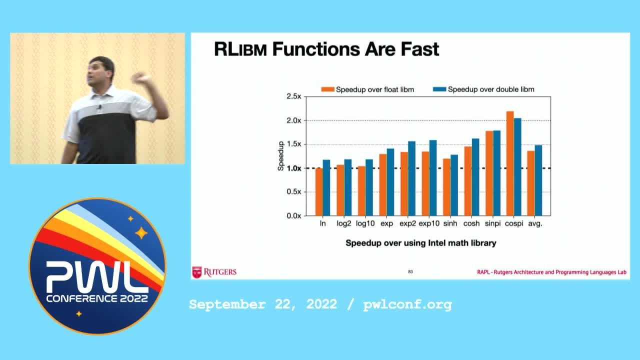 2X. So I would encourage you to test it out. So we are like faster. So the moral of the story, like we are not only correct but also fast, That shows the value of the idea. So it's just like four of us building this library. 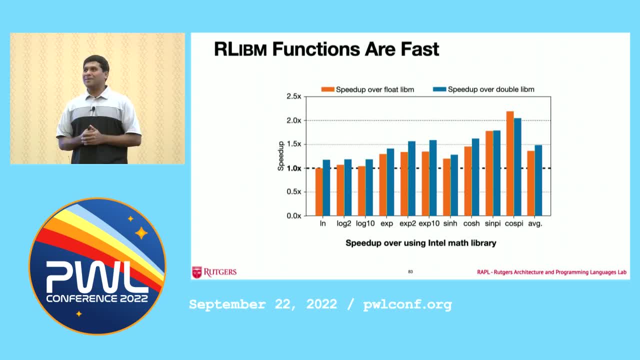 So I don't have an army of engineers. I don't have engineers building this right. So, in contrast, many production companies have teams of 30, 40 people building these libraries. Imagine how much faster we can go if you had a team of that size. 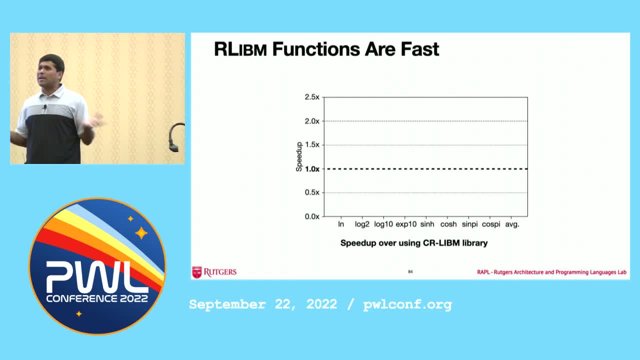 So now the last thing I want to demonstrate is like: how do we compare to correctly rounded libraries, CRLibm? In contrast to CRLibm, we are close to 2X faster on average across all functions. Okay, So all this is great. 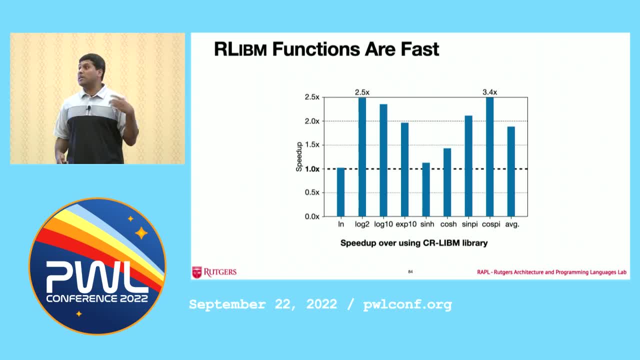 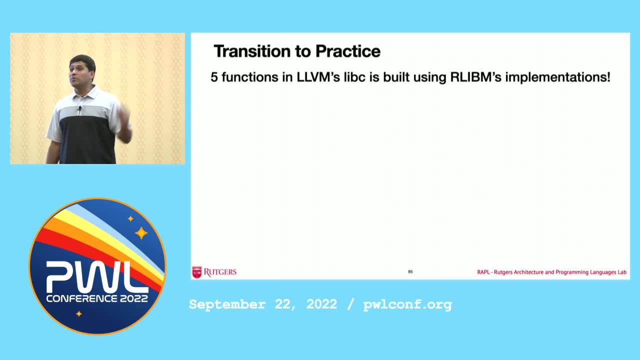 Like even with a small team, we have been pushing these functions into the library. Okay, So we have been collaborating with the LLVM developers and pushing some of these functions into the new Libm that the LLVM is developing. So five of these functions have been incorporated into LLVM's new Libm, which are correctly. 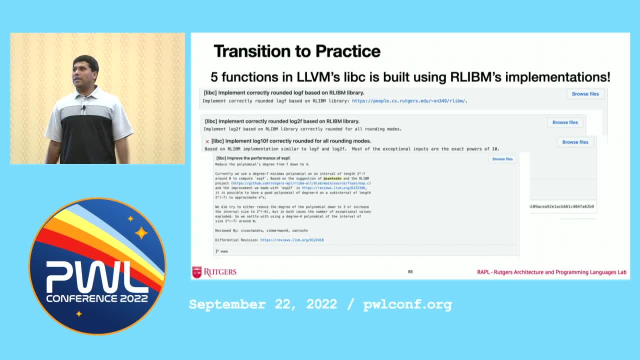 rounded for all rounding modes. Again, Q Li has been instrumental and Paul Zimmerman from France also has been helping us out in this effort. So I think like if we are successful in the next standard which happens in the next year, which is supposed to come out in 2029,, we want to give enough evidence for IEEE standards. 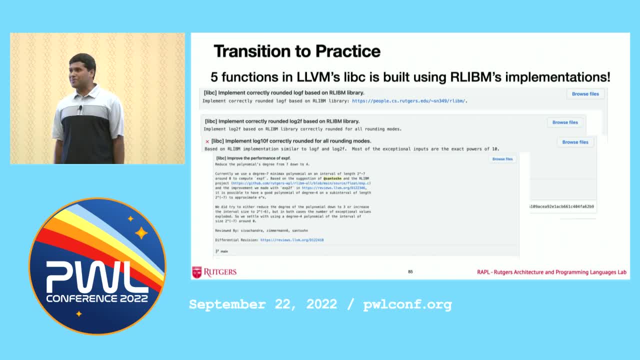 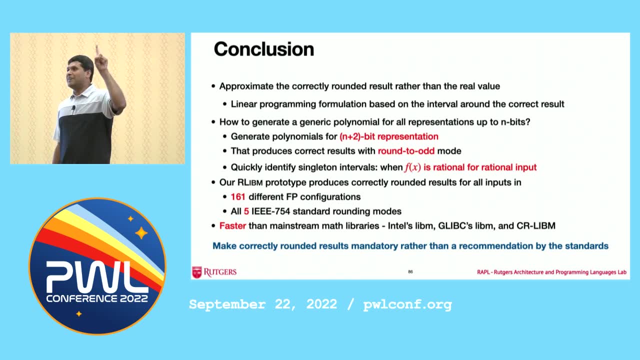 committee to mandate correct rounding, at least for 32 bits. Okay, So, to conclude, what are the four takeaways that I want? One: directly approximate the correctly rounded result. There is an interval of real values around the correctly rounded result. Produce any value, you're good.